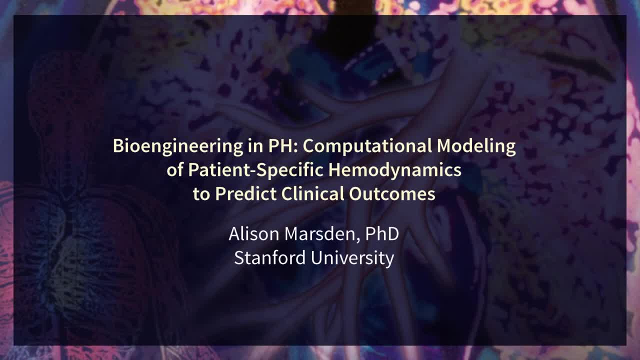 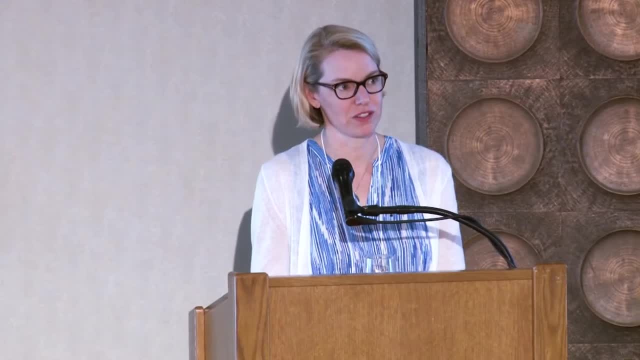 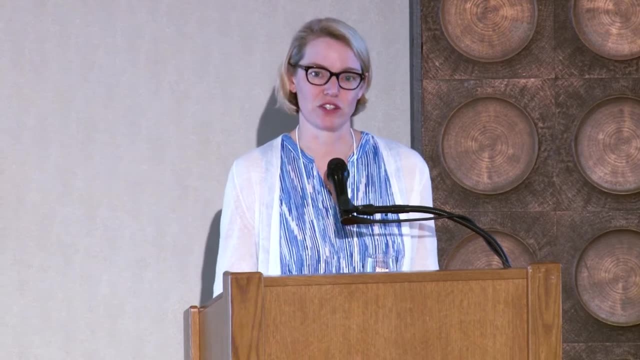 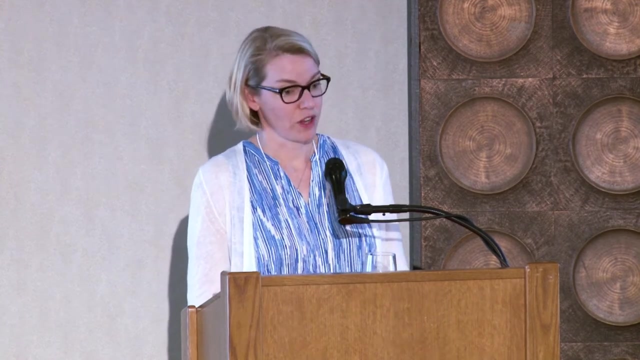 Okay, so I run a lab that we work on computational modeling of blood flow in the cardiovascular system and since I came back to Stanford a couple of years ago, we have been we've started to take an interest in assessing the hemodynamics in pulmonary hypertension patients And part 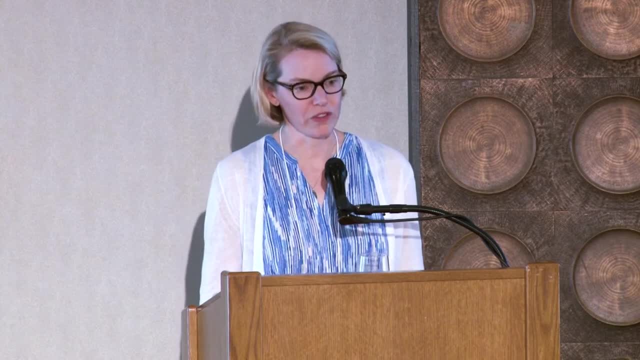 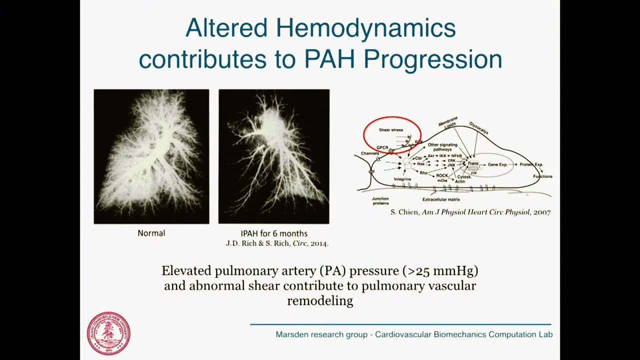 of our motivation for doing this is that we know very well that altered hemodynamics is a contributor to pH progression and, particularly thinking about the elevated pulmonary pressures, together with abnormal wall shear stress conditions, we'd like to have a better understanding of how those hemodynamics contribute to vascular remodeling And, in particular, we've really 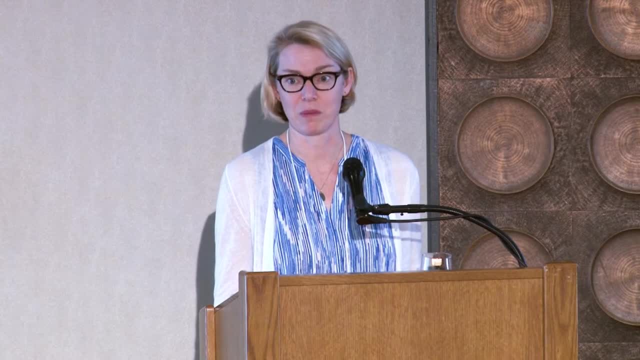 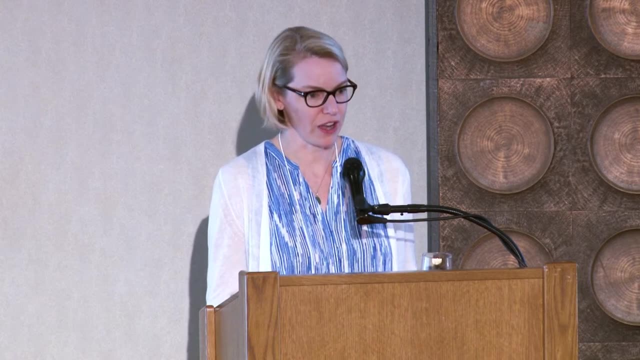 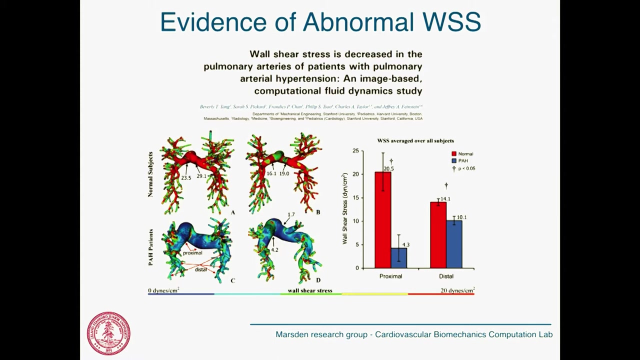 taken a step back and started to ask the question: what are the hemodynamic conditions in these patients, Really thinking about a couple of different categories? So, just to review, there is evidence that hemodynamics is abnormal in the pulmonary arteries of pH patients And primarily that's been looked at in the 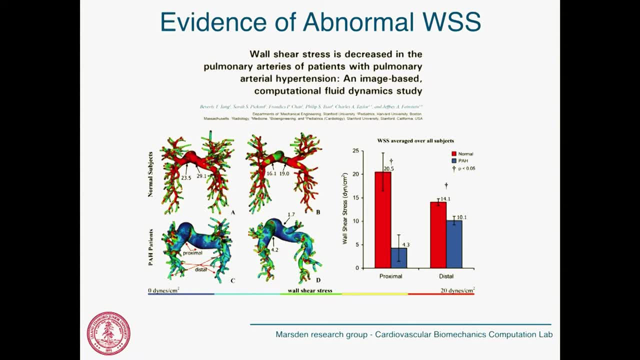 proximal pulmonary arteries. So there have been prior studies done here at Stanford. This is a study by Bev Tang together with Charlie Taylor and Jeff Feinstein, And they're looking primarily at the MPA and then the branch PAs, showing that the wall 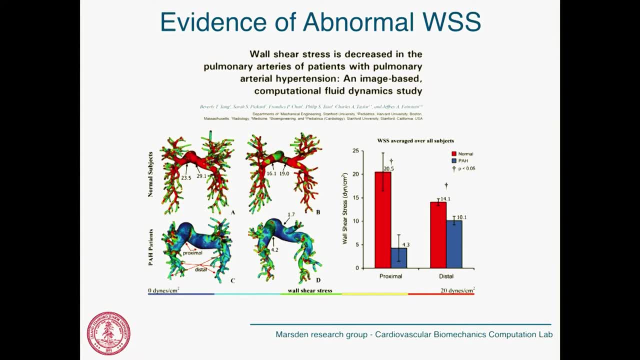 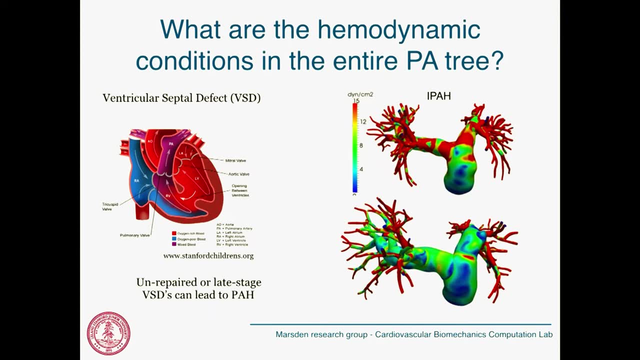 shear stress was significantly decreased in the MPA, in pH, compared to normal. And continuing from that, we wanted to then sort of take this a step further and ask: what are the hemodynamic conditions, not only in the proximal arteries but looking down the entire pulmonary? 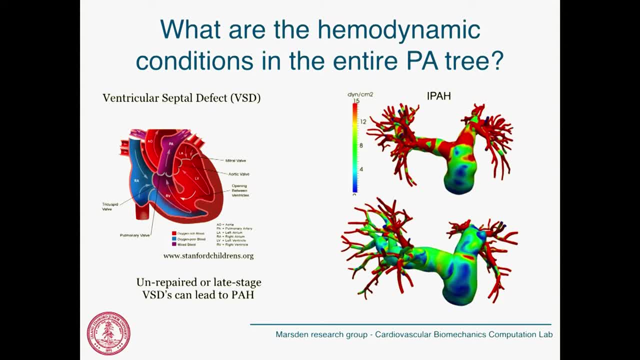 tree. And then looking at two categories of patients who develop pH, the first being patients who develop pH secondary to congenital heart disease, For example, patients with late or unrepaired VSD, And then also in patients with IPH, looking at how the hemodynamics changes with disease. 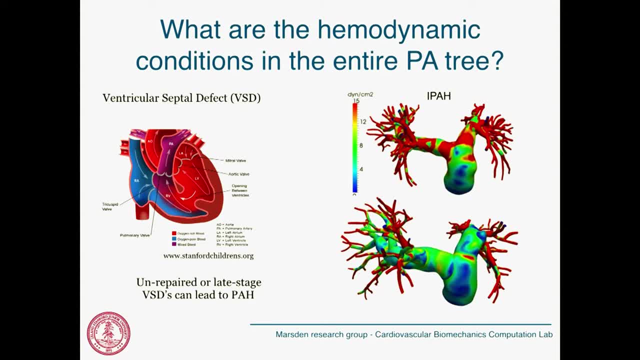 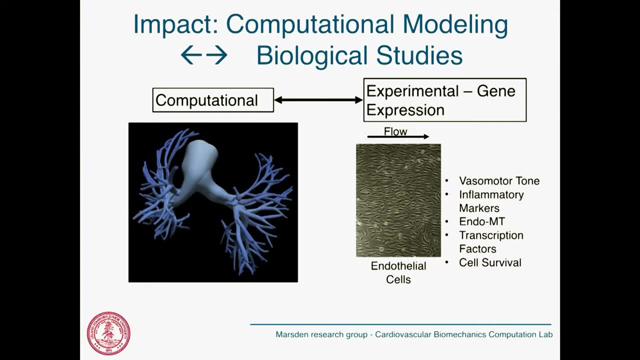 progression, And so we're using a computational modeling approach to do this. So using computational modeling, where we construct patient-specific models directly from the image data, usually CT or MRI, And then part of our motivation for this is also really wanting to make sure that we're 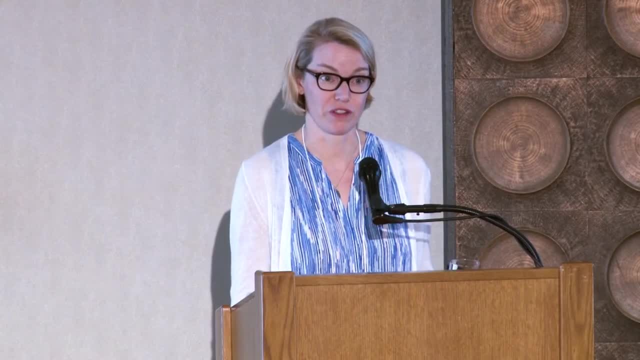 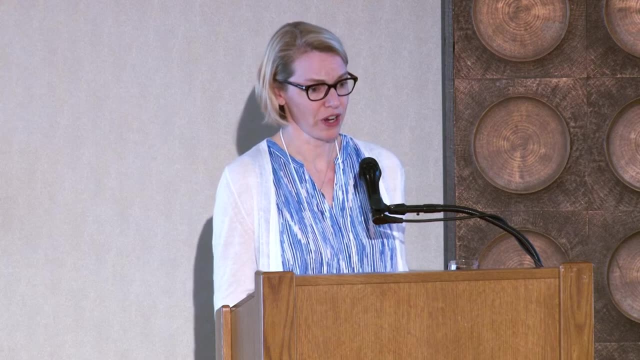 doing the right experiments when we go to the lab and look at endothelial shear stress, And so we've been collaborating with Marlene Rabinovich on that front and trying to really directly use some of the mechanical data that we're getting, particularly on wall shear. 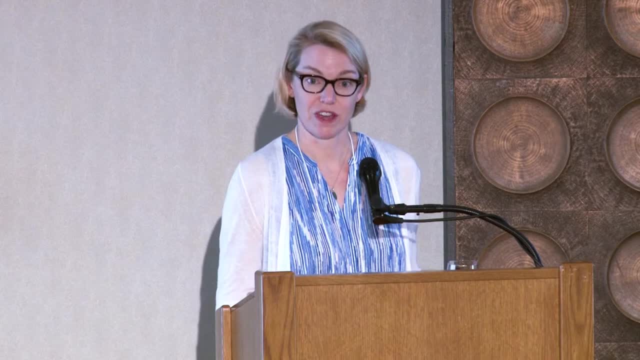 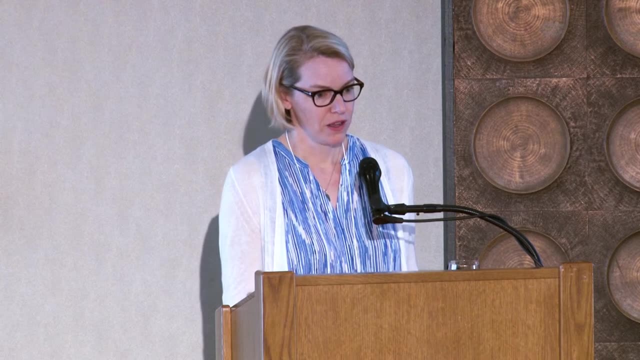 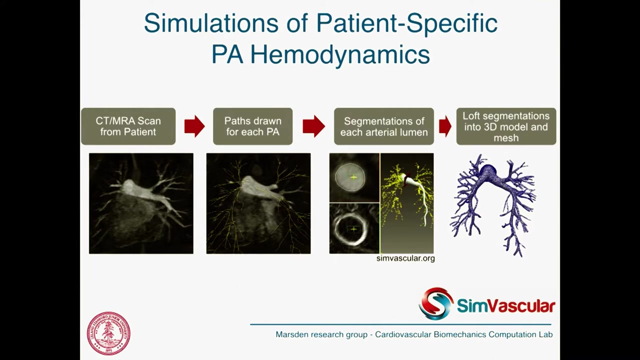 stress and using that to drive sort of more precise endothelial shear experiments where we can look at gene expression. Our computational methods are typically starting from a CT or MRI scan of a pH patient. We then draw centerline paths down the vessels. All of the processes are done through CT. 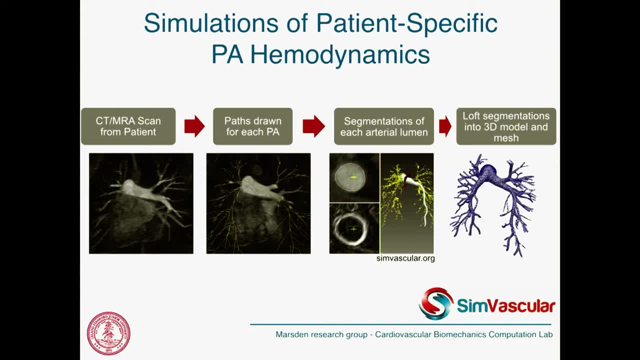 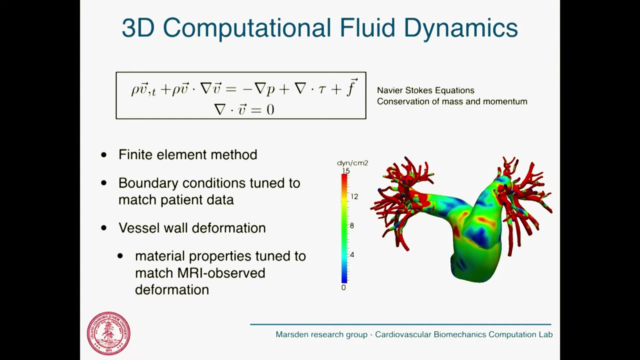 pulmonary vessels that we can reasonably see in the image data. we segment the lumen and we construct a pretty complex three-dimensional computer model of the pulmonary vasculature that looks like this: we then use three-dimensional computational fluid dynamics to model flow in these 3d models, the 3d CFD. 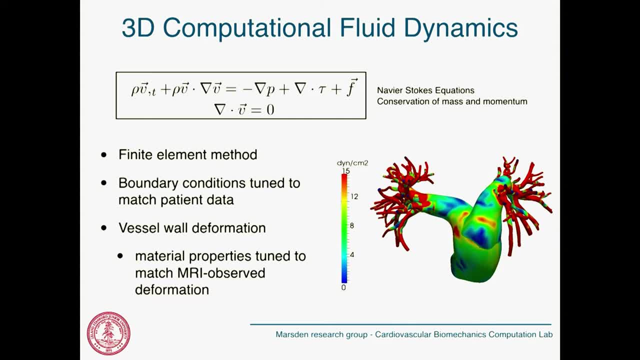 models are really used to model the proximal PAs, so generally all the vessels that we can see in a CT scan, down to about one millimeter in diameter, and just to remind everybody. so the equations that we're solving are really just the conservation of mass and momentum of the fluid going through the 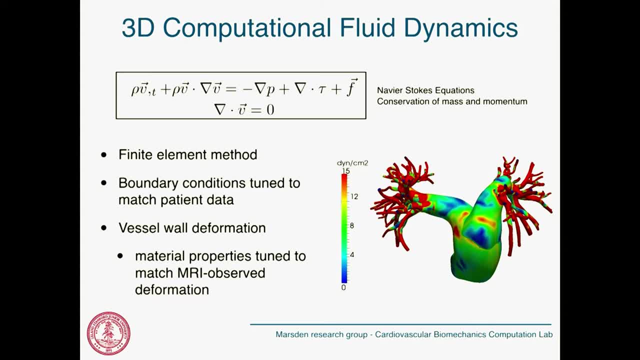 model. we kind of borrow a lot of techniques that have been developed in more traditional engineering fields to use a finite element of the fluid that we can see in a CT scan. and we kind of borrow a lot of techniques that have been developed in more traditional engineering fields to use a finite element. 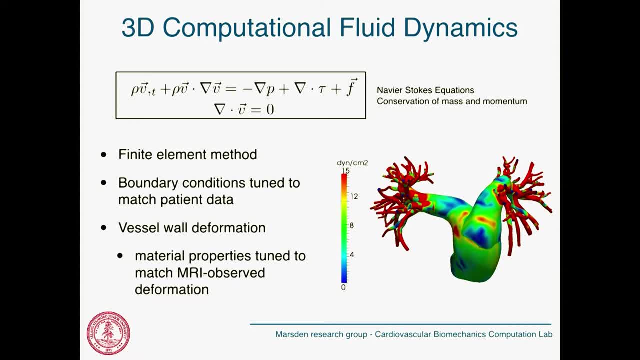 method to solve these equations. for each model, we tune the inlet and outlet boundary conditions to match a set of clinical data that's been collected for each of our patients, and we do include vessel wall deformation in our models and, where possible, we match or we tune the material properties such that we 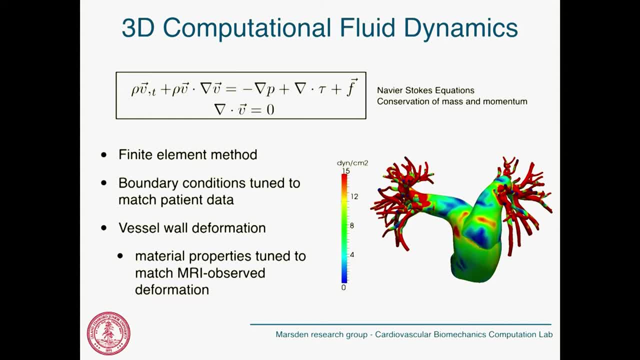 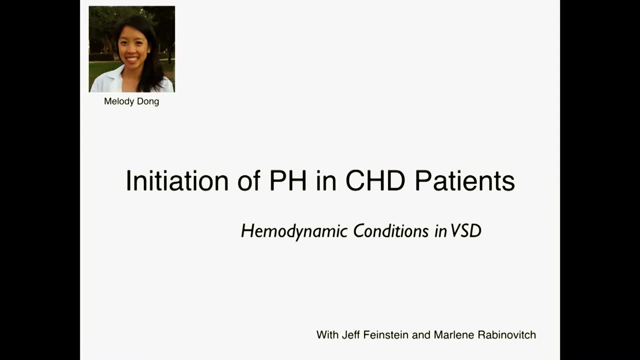 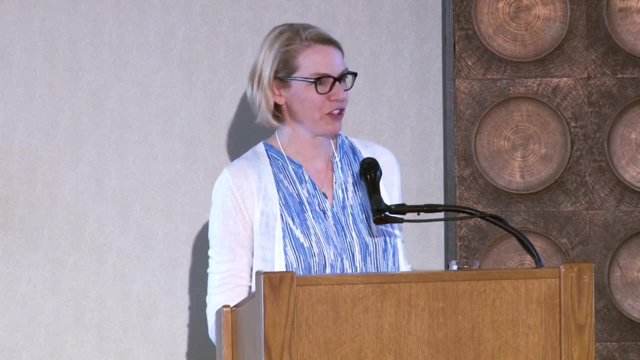 match, for example, deformation in the MPA that's observed or measured in MRI. so we've really looked at two groups of patients here, and the two people who've done all of this work are sitting in the back, so we can also feel free to bother them for additional details. so this first project was done by Melody Dong. 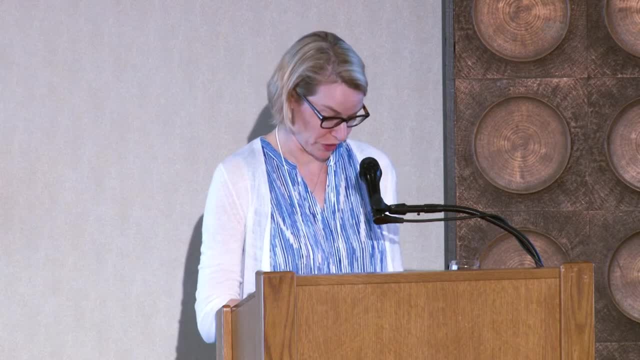 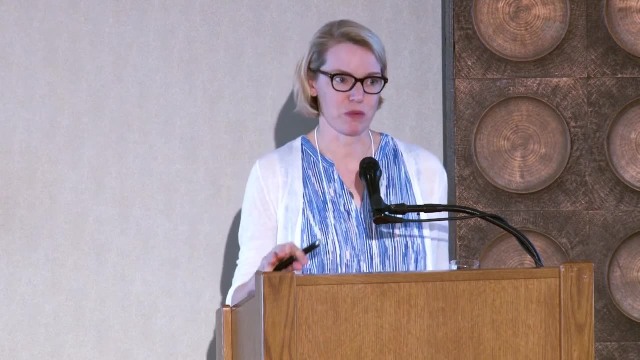 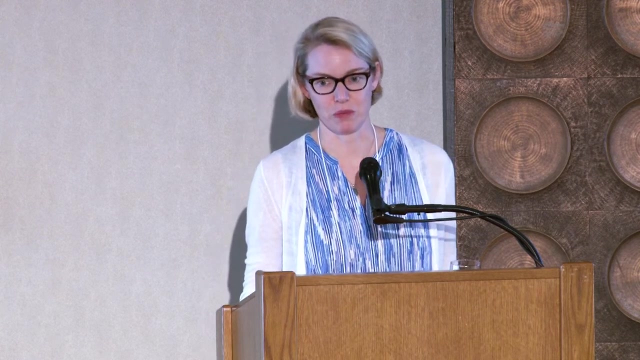 some of these results are still still preliminary. we're just still getting started on some of this, but our goal here was really to try to separate out and ask in a patient with, for example, an unrepaired VSD, what are the hemodynamic conditions in the PAs that may lead to initiation of? 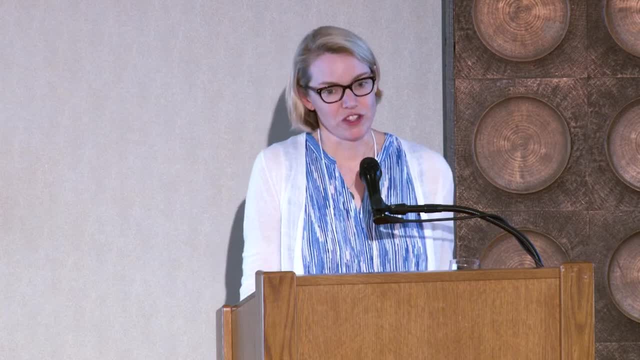 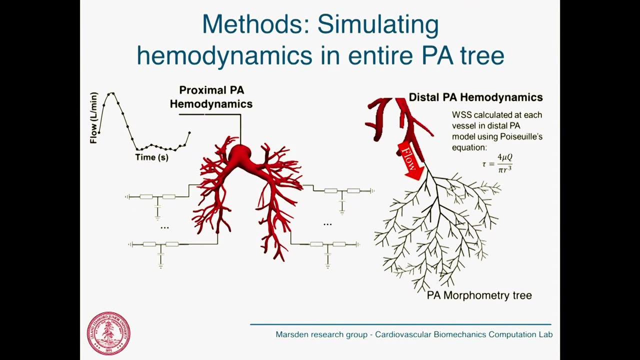 pH in these patients, and so we took kind of a two-step approach here. we wanted to model both the hemodynamics and the proximal PAs as well as in the distal tree, and so we use the 3d modeling approach that I just told you about. 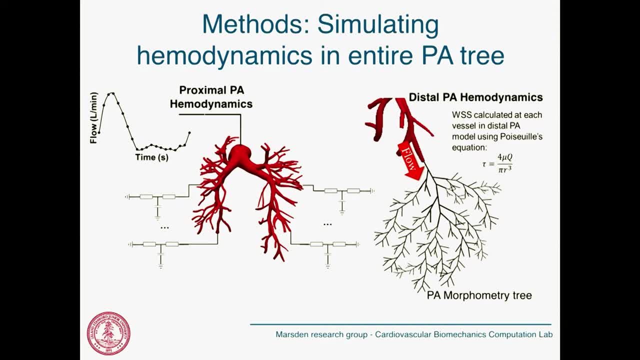 building a model directly from the CT scan to examine the flow in the proximal vessels and then at the end of the process we're going to look at the outlet of each of these are. at each outlet in the model here we then construct a distal, a morphometric tree of the distal vasculature. so we'd like to 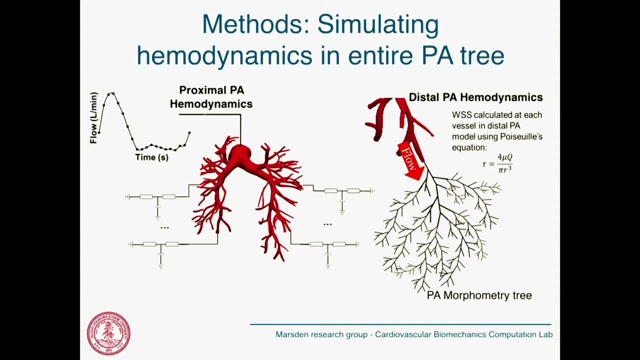 be able to use then the 3d model to get the proximal vessels and then this morphometric tree to get the entire distal tree. downstream of that we solve the 3d model directly with CFD and then the distal tree we make a quasi. 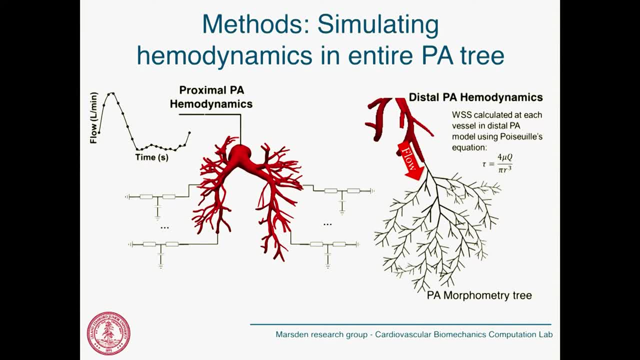 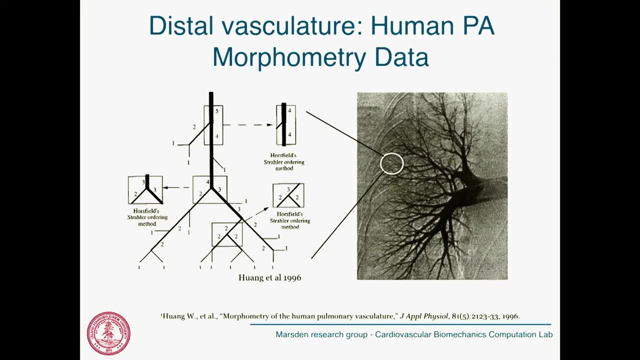 assumption. so we assume a parabolic flow profile and compute an estimate of the shear stress in all of those vessels downstream. the morphometric trees for right now are constructed from this 96 paper by Wong. these are more. this is a morphometric data set for an adult. 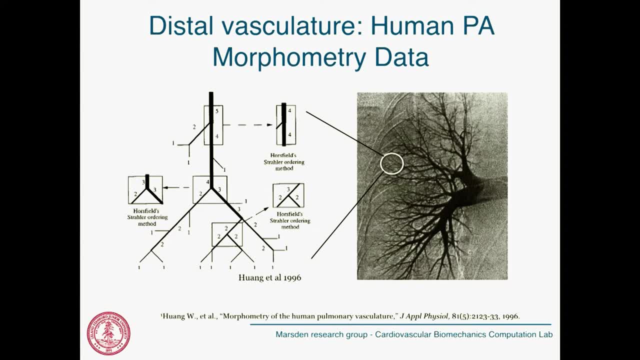 normal pulmonary tree for the case of the disease pH patients that you'll see later in this video. and then we're going to use the 3d model to get the 3d model and compute an estimate of the shear stress in all of those vessels downstream. 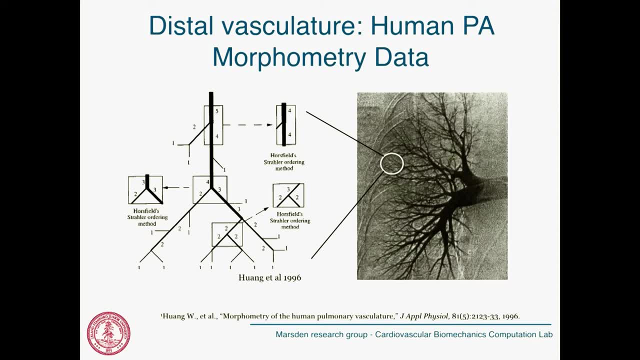 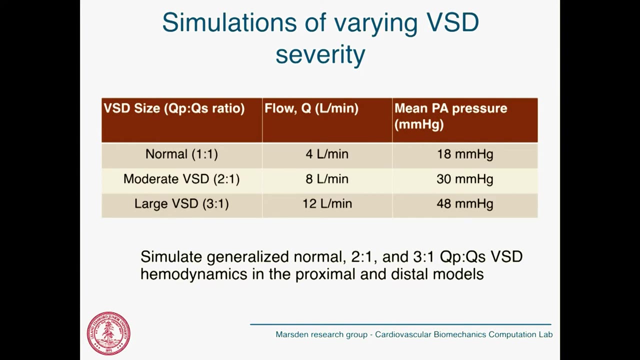 on. we have also been able to adapt this tree to do the kind of pruning that we see in pH, and we're currently investigating ways to scale this data for younger patients, such as infants. so the first results that I'll show you are a normal pulmonary model, where we've then artificially altered the inlet. 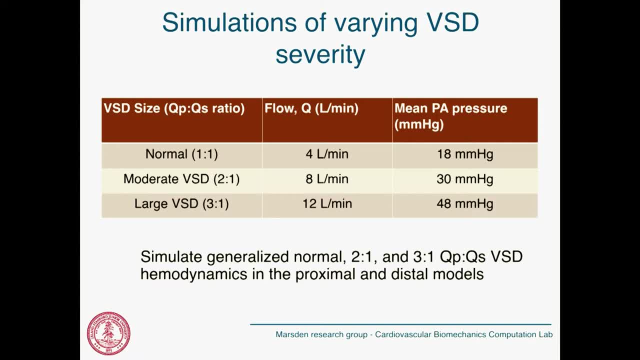 conditions to account for or to model the case of a normal patient and then a two-to-one, and a two-to-one patient and then a two-to-one patient and then a three-to-one VSD flow conditions. so these are the flow rates that you see. 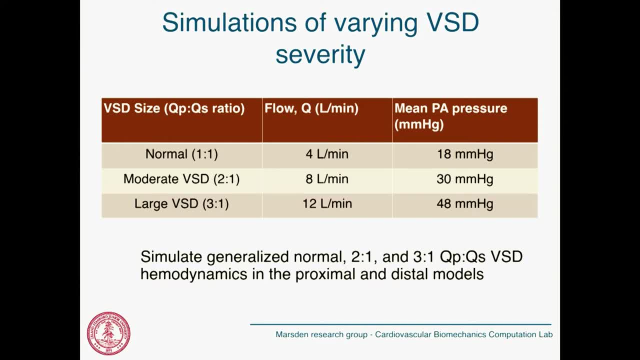 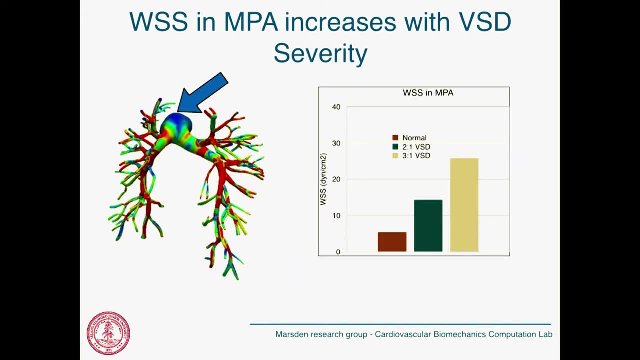 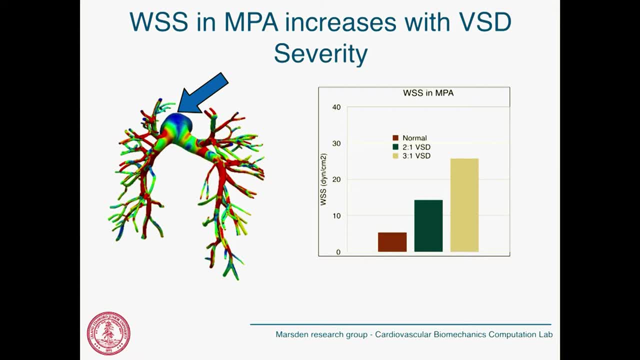 with. we're going to look at the MPA to start with. we're going to look at the MPA to start with. the shear stress increases from about five. with the shear stress increases from about five with. the shear stress increases from about five to about 25 as you increase the flow. 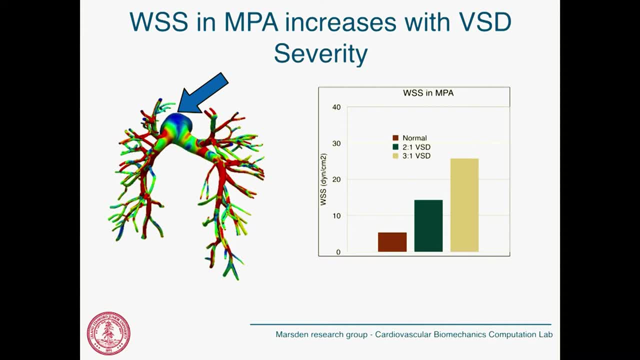 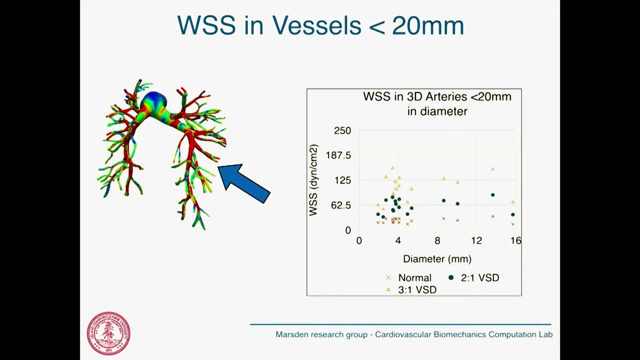 to about 25, as you increase the flow to about 25, as you increase the flow rate from normal to a three-to-one VSD rate, from normal to a three-to-one VSD rate, from normal to a three-to-one VSD, as you travel down to arteries that are. 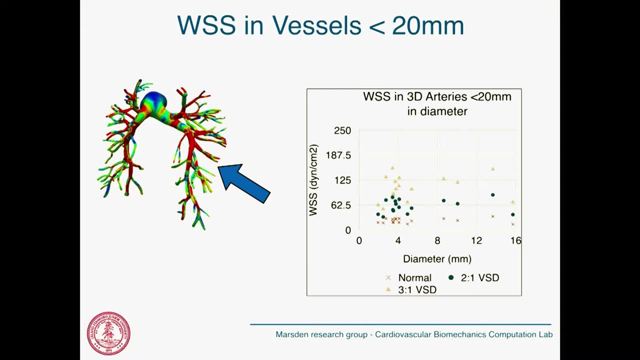 as you travel down to arteries that are, as you travel down to arteries that are less than 20 millimeters in diameter- we less than 20 millimeters in diameter, we less than 20 millimeters in diameter- we start to see more significant, start to see more significant. 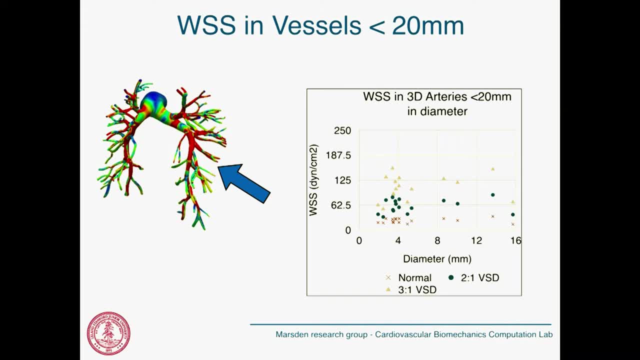 start to see more significant elevations in shear stress. so going elevations in shear stress, so going elevations in shear stress. so going from roughly 20 to 30 in the normal, from roughly 20 to 30 in the normal, from roughly 20 to 30 in the normal models that are shown by these red X's. 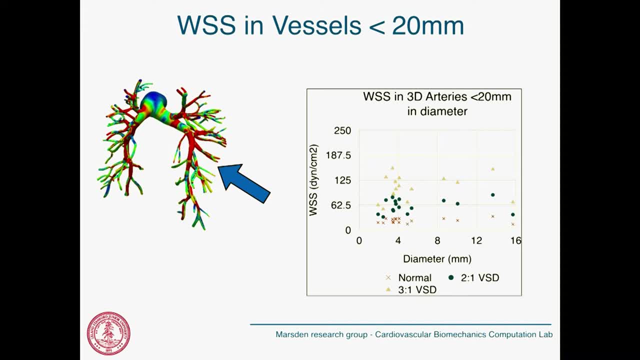 models that are shown by these red X's, models that are shown by these red X's to say on the order of 50 or 60 for the, to say on the order of 50 or 60 for the, to say on the order of 50 or 60 for the two to one VSD, and then getting closer. 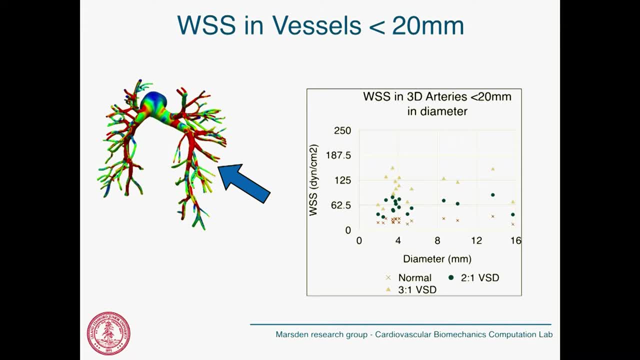 two to one VSD and then getting closer- two to one VSD, and then getting closer to a range of a hundred for the three to to a range of a hundred for the three to to a range of a hundred for the three to one VSD. so we're starting to see some. 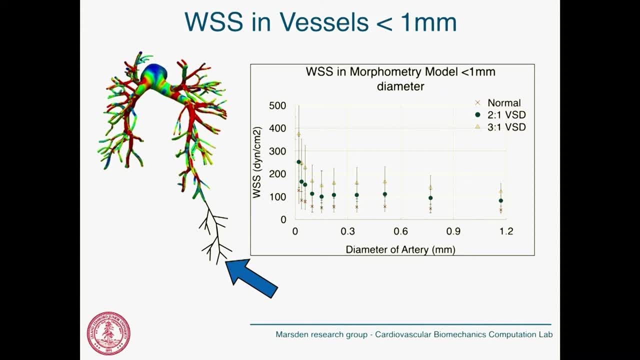 one VSD. so we're starting to see some one VSD. so we're starting to see some fairly elevated shear stress values, at fairly elevated shear stress values, at fairly elevated shear stress values, at these higher flow rates and then going, these higher flow rates and then going. 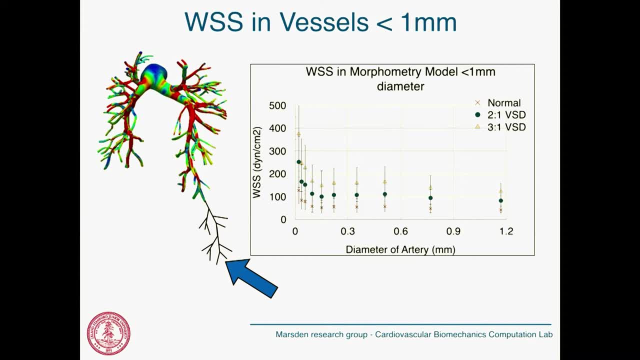 these higher flow rates and then going to in the morphometric tree vessels, less to in the morphometric tree vessels, less to in the morphometric tree vessels, less than one millimeter, where of course it's than one millimeter, where of course it's than one millimeter, where of course it's thought that the disease originates you. 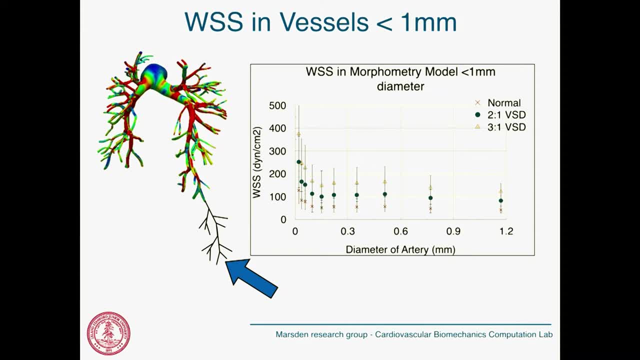 thought that the disease originates. you thought that the disease originates. you can see that as we go smaller in can see that as we go smaller in, can see that as we go smaller in diameter, we really start to get some diameter. we really start to get some diameter. we really start to get some severely elevated shear stress values in. 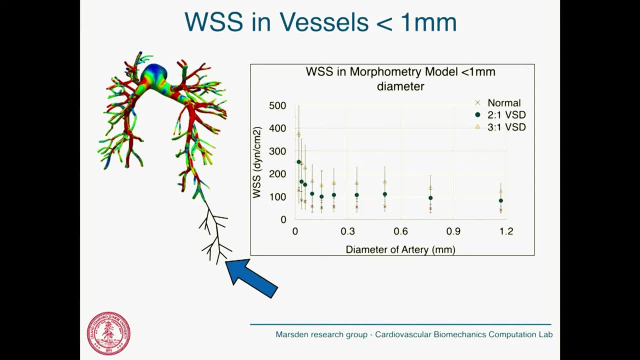 severely elevated shear stress values, in severely elevated shear stress values in those distal PAS. so we're looking at those distal PAS. so we're looking at those distal PAS. so we're looking at values upwards of a hundred two hundred, values upwards of a hundred two hundred. 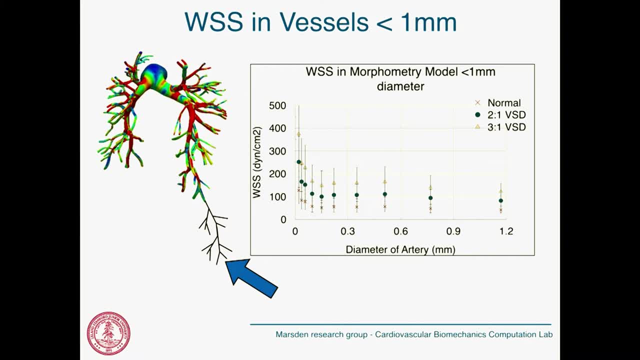 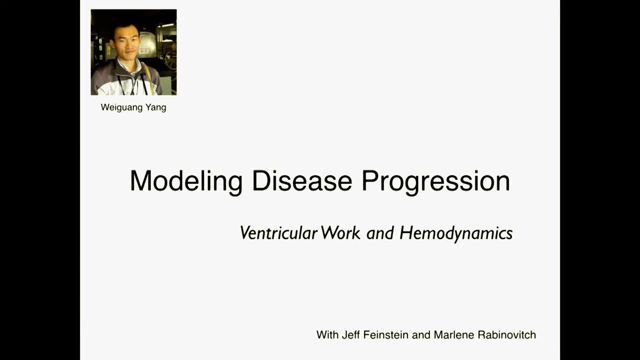 values upwards of a hundred two hundred dynes per centimeter squared, we went we. dynes per centimeter squared, we went. we. dynes per centimeter squared, we went. we then wanted to go on and look at, then wanted to go on and look at, then wanted to go on and look at patients who have pH. how did these? 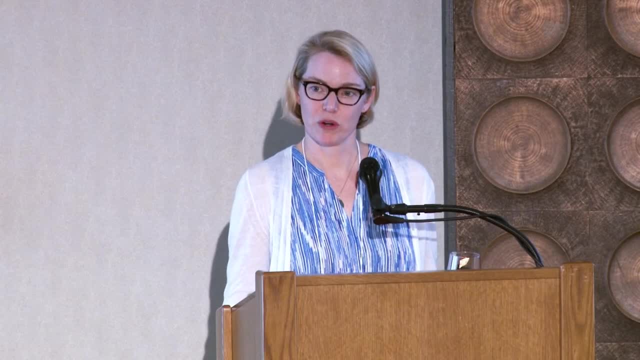 patients who have pH. how did these patients who have pH, how did these hemodynamic conditions change over? the hemodynamic conditions change over the hemodynamic conditions change over the course of disease and, in particular, we course of disease and, in particular, we course of disease? and, in particular, we wanted to use computational modeling for 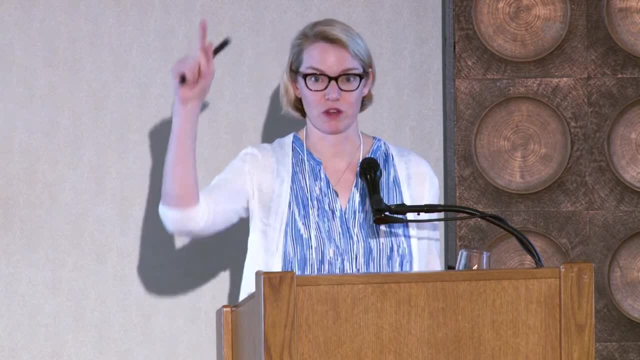 wanted to use computational modeling for. wanted to use computational modeling for two different goals. the first thing: I'm two different goals. the first thing, I'm two different goals. the first thing I'm going to tell you about which was done. going to tell you about which was done. 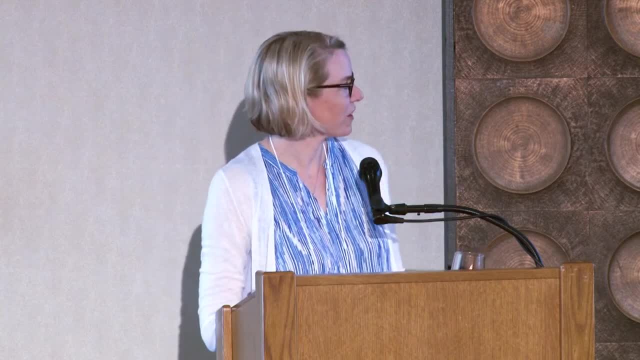 going to tell you about, which was done by way. guang, who's also sitting in the by way. guang, who's also sitting in the by way. guang, who's also sitting in the back. there was to look at whether we back. there was to look at whether we. 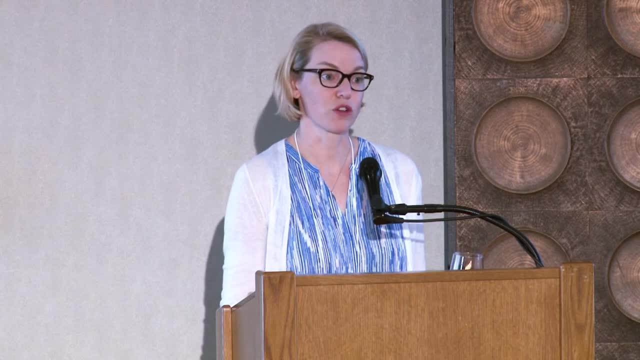 back there was to look at whether we could use a simple computational model. could use a simple computational model, could use a simple computational model of ventricular work. so right, ventricular of ventricular work, so right, ventricular of ventricular work, so right, ventricular stroke work to predict disease. 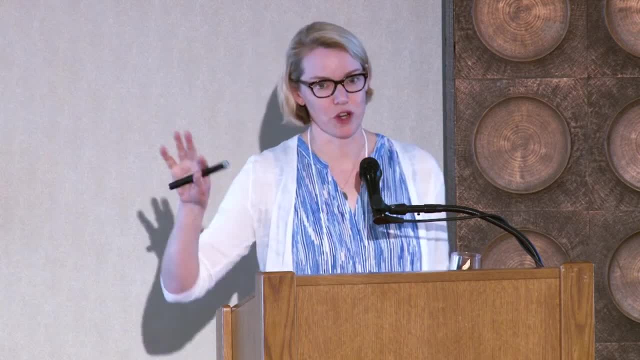 stroke work to predict disease. stroke work to predict disease progression or clinical worsening in progression or clinical worsening in progression or clinical worsening in these patients, and then we'll talk more these patients, and then we'll talk more these patients, and then we'll talk more about. go back to the tree- hemodynamics. 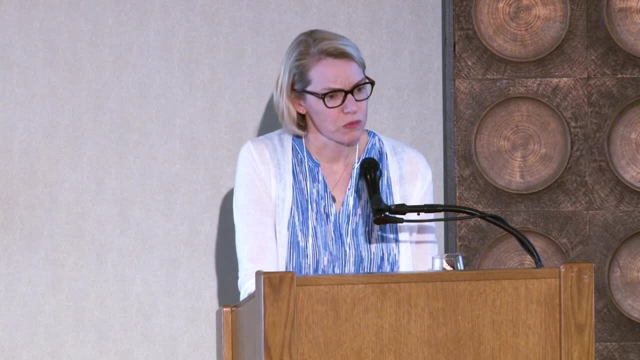 about go back to the tree hemodynamics, about go back to the tree hemodynamics and look at shear stress. so we, we all, and look at shear stress. so we, we all, and look at shear stress. so we, we all, know that stroke work is the area, know that stroke work is the area. 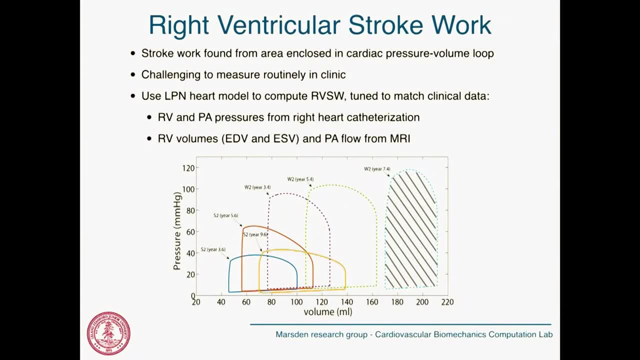 know that stroke work is the area enclosed inside of a pressure-volume loop, enclosed inside of a pressure-volume loop, enclosed inside of a pressure-volume loop of the heart. and so we had this idea of the heart. and so we had this idea of the heart, and so we had this idea that we could artificially produce a PV. 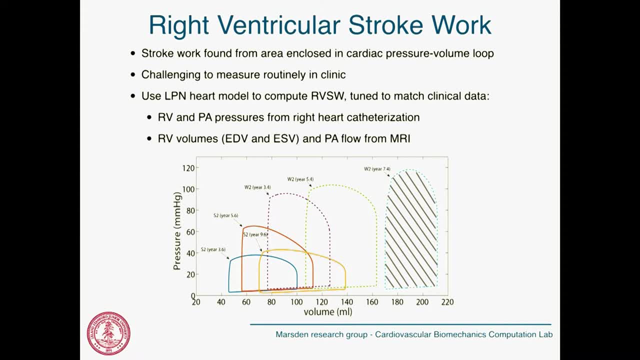 that we could artificially produce a PV, that we could artificially produce a PV loop using a computational model. so just a loop using a computational model. so just a loop using a computational model. so just a simple circuit. lump parameter model of simple circuit. lump parameter model of simple circuit. lump parameter model of the right ventricle. and so we decided to. 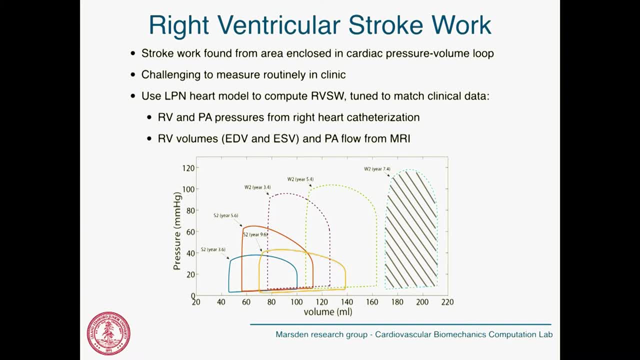 the right ventricle, and so we decided to the right ventricle, and so we decided to collect from the Packard database. collect from the Packard database. collect from the Packard database, working with Jeff Feinstein, a set of working with Jeff Feinstein, a set of. 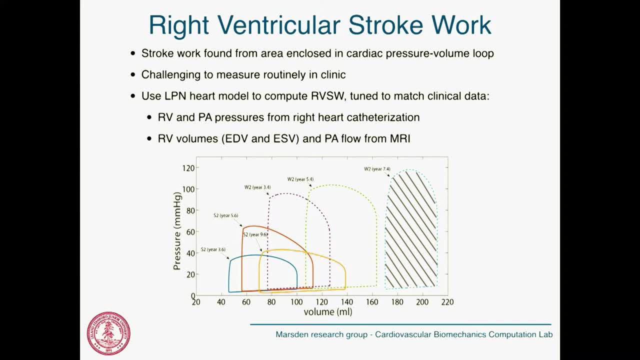 working with Jeff Feinstein, a set of data for patients with pH over, who had data for patients with pH over, who had data for patients with pH over, who had both MRI and cath at multiple time, both MRI and cath at multiple time, both MRI and cath at multiple time points, and and we thought, well, we could. 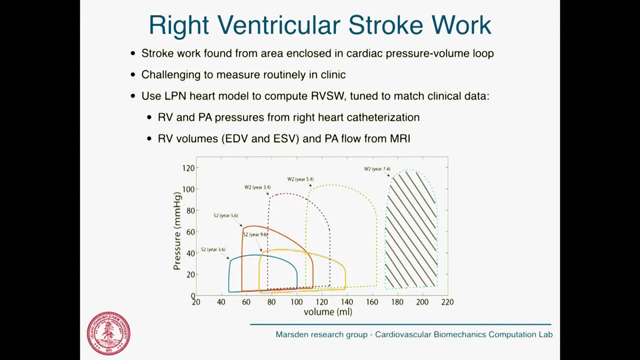 points and and we thought well, we could points and and we thought well, we could evaluate the right ventricular stroke, evaluate the right ventricular stroke, evaluate the right ventricular stroke work and see if this is predictive of work, and see if this is predictive of work and see if this is predictive of clinical worsening in these patients. so 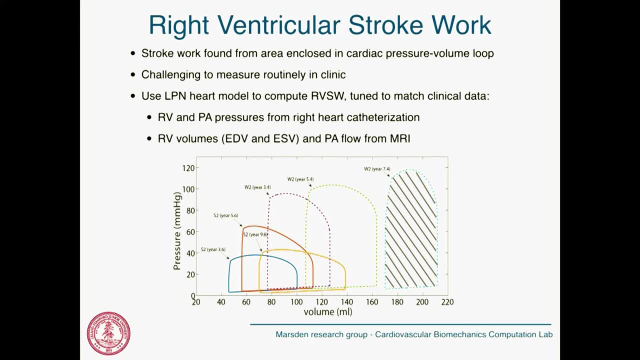 clinical worsening in these patients. so clinical worsening in these patients. so for each patient, we used a lump. for each patient, we used a lump. for each patient, we used a lump parameter heart model to compute the parameter heart model. to compute the parameter heart model to compute the right ventricular stroke work, we tuned. 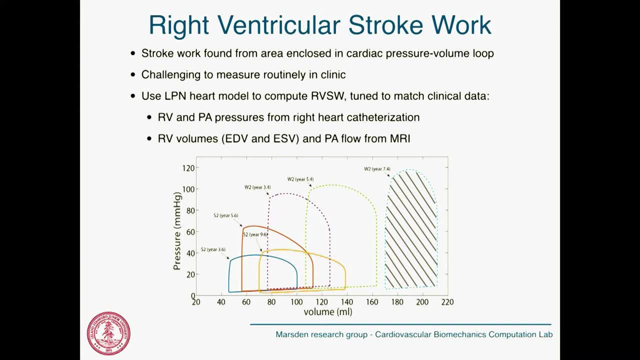 right ventricular stroke work. we tuned right ventricular stroke work. we tuned the heart model to match the clinical, the heart model to match the clinical, the heart model to match the clinical data collected for the patient. and we data collected for the patient and we data collected for the patient and we use both RV and PA pressures from right. 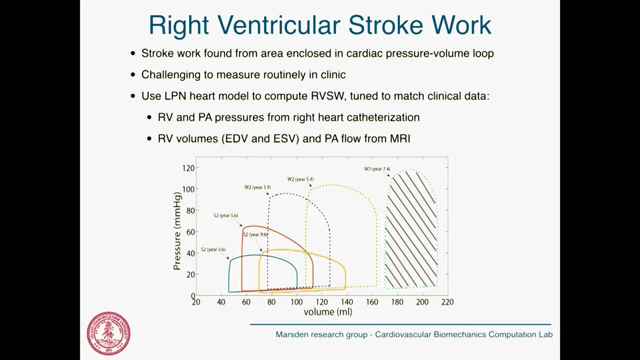 use both RV and PA pressures from right. use both RV and PA pressures from right heart cath, as well as RV volumes and PA heart cath, as well as RV volumes and PA heart cath, as well as RV volumes and PA flow from MRI. to tune the model. the 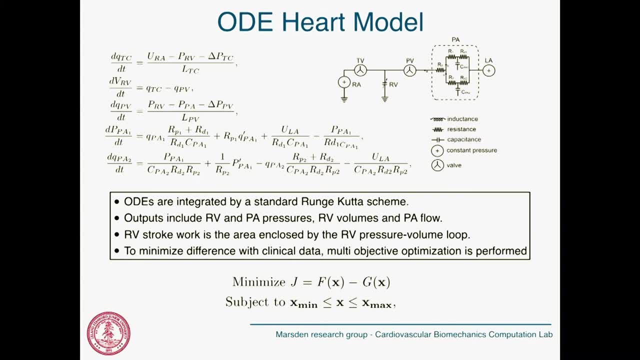 flow from MRI to tune the model. the flow from MRI to tune the model. the model looks like this: so it's a circuit model. looks like this: so it's a circuit model. looks like this: so it's a circuit. the elements of the circuit are governed. the elements of the circuit are governed. 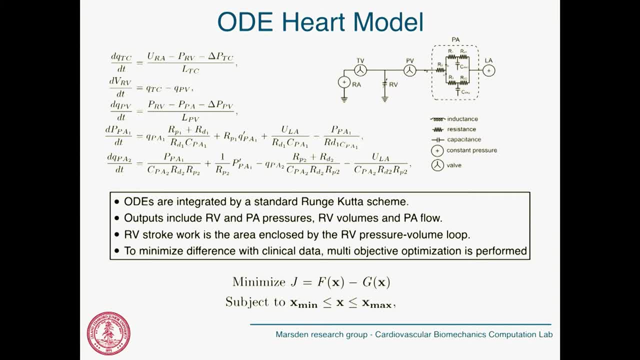 the elements of the circuit are governed, governed by a set of ordinary, governed by a set of ordinary, governed by a set of ordinary differential equations. we can integrate differential equations. we can integrate differential equations. we can integrate these in a, in a simple code, like in these in a, in a simple code, like in: 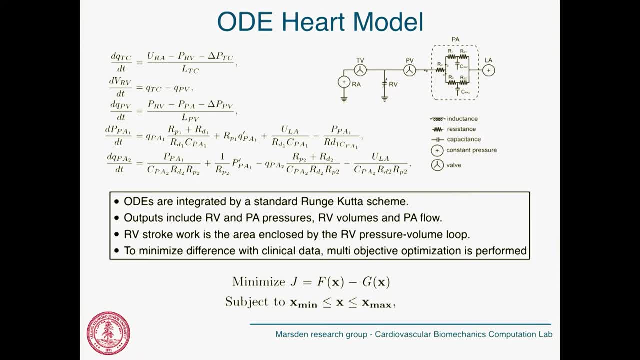 these in a, in a simple code, like in MATLAB, and the outputs of this are MATLAB and the outputs of this are MATLAB. and the outputs of this are basically the PV loop, where we can basically the PV loop, where we can basically the PV loop where we can compute the RV stroke work in order to 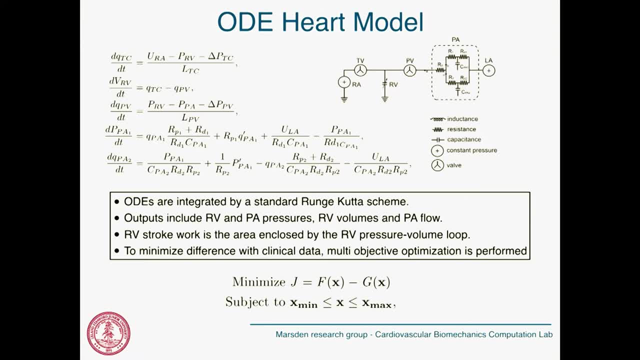 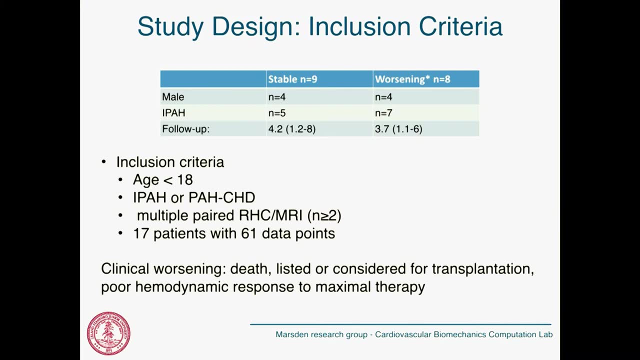 compute the RV stroke work. in order to compute the RV stroke work, in order to tune the model to match the clinical tune. the model to match the clinical tune. the model to match the clinical data. we performed an optimization method. data. we performed an optimization method. data. we performed an optimization method and in the study we had 17 patients with 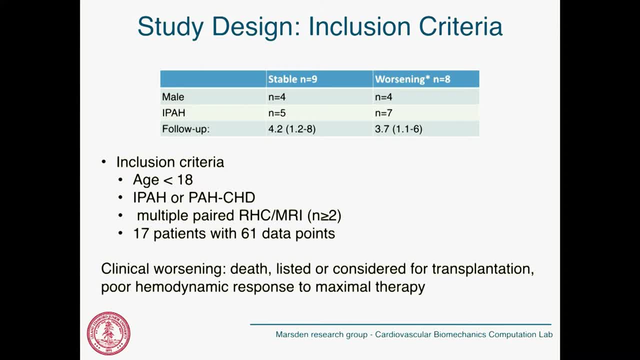 and in the study we had 17 patients with and in the study we had 17 patients with a total of 61 data points. because each a total of 61 data points, because each a total of 61 data points, because each patient had multiple time points that we 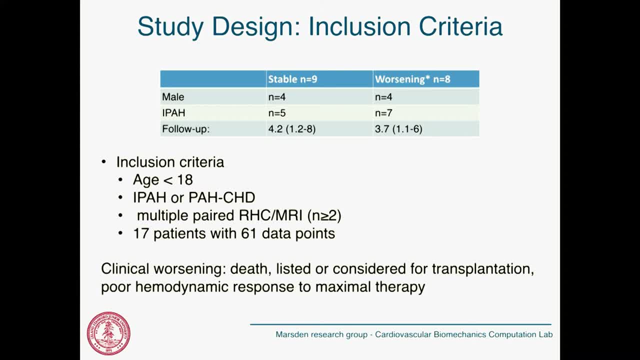 patient had multiple time points that we patient had multiple time points that we looked at. these were all patients under looked at. these were all patients under looked at. these were all patients under 18 who had IPA H or pH. 18 who had IPA H or pH. 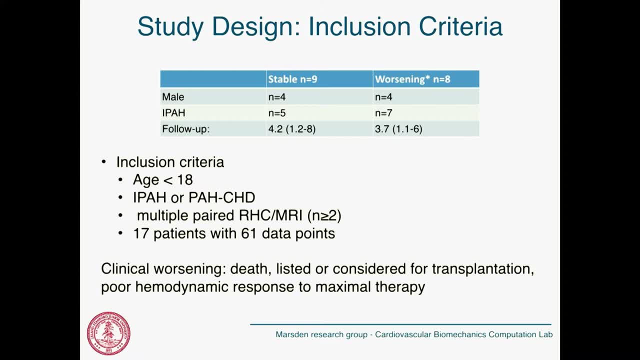 18 who had IPA H or pH due to congenital heart disease, and we due to congenital heart disease, and we due to congenital heart disease, and we classified these into a stable group and classified these into a stable group. and classified these into a stable group and a worsening group and so we had, I think, 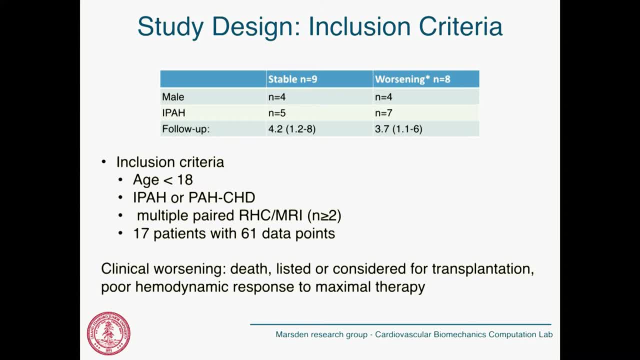 a worsening group, and so we had, I think, a worsening group, and so we had, I think, five in the stable group and seven in five in the stable group and seven in five in the stable group and seven in the worsening group. we defined clinical the worsening group. we defined clinical. 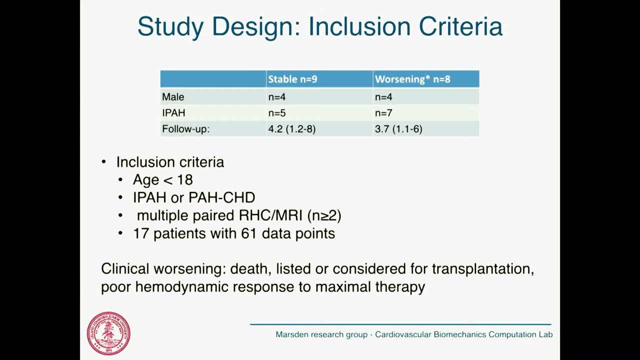 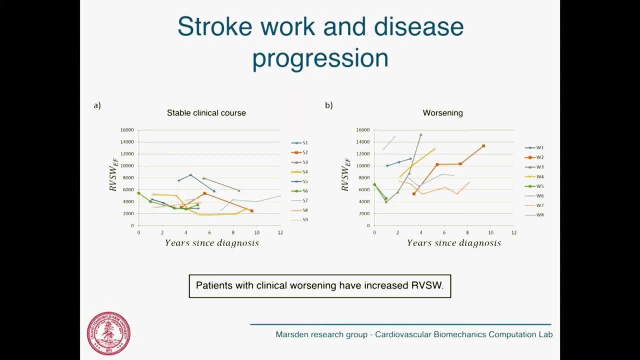 the worsening group, we defined: clinical worsening as death listed or considered worsening as death listed or considered worsening as death listed or considered for transplantation or poor hemodynamic for transplantation or poor hemodynamic for transplantation or poor hemodynamic response to maximal therapy and response to maximal therapy. and. 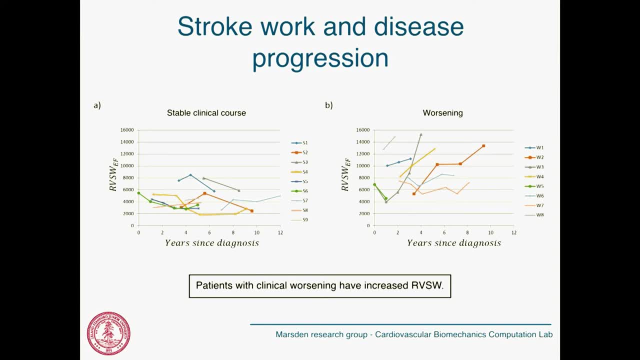 response to maximal therapy, and so this is just to give you a qualitative. so this is just to give you a qualitative, so this is just to give you a qualitative idea of how their RV stroke work changes, idea of how their RV stroke work changes, idea of how their RV stroke work changes over over the years of since diagnosis. 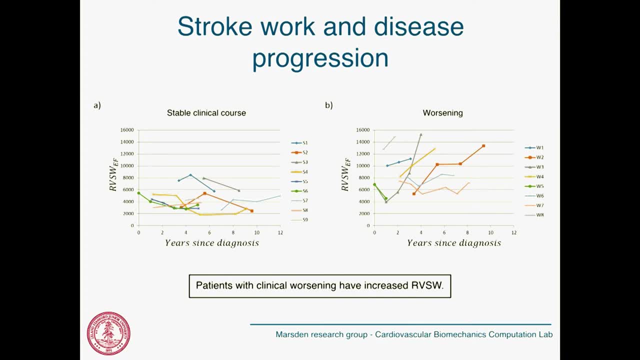 over over the years of since diagnosis, over over the years of since diagnosis for these patients. so you can see that for these patients. so you can see that for these patients, so you can see that the paint for the patients who had a, the paint for the patients who had a, 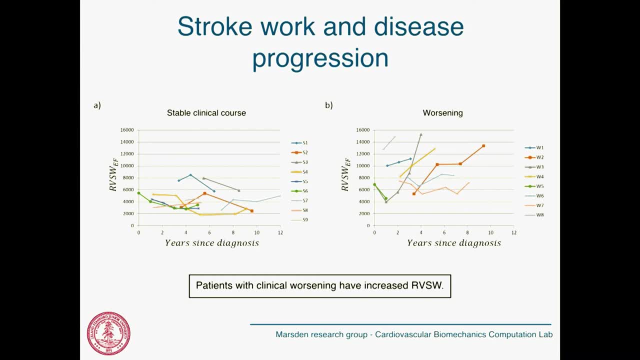 the paint. for the patients who had a relatively stable clinical course: their relatively stable clinical course: their relatively stable clinical course: their RV stroke work remained relatively RV stroke work remained relatively RV stroke work remained relatively stable, usually over several years. stable, usually over several years. stable, usually over several years. however, the patients that were classified: 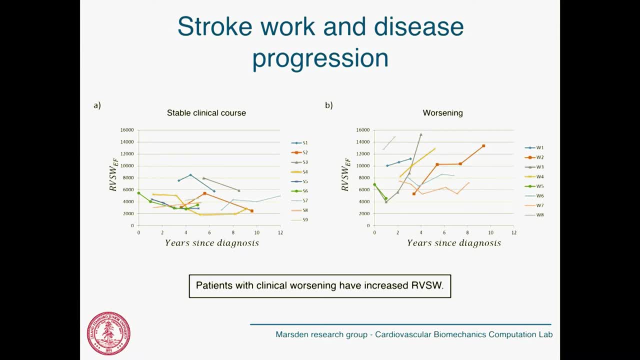 however, the patients that were classified, however, the patients that were classified in the clinical worsening group in the clinical worsening group, in the clinical worsening group generally had RV stroke work values that generally had RV stroke work values, that generally had RV stroke work values that climbed quite steeply and also were on. 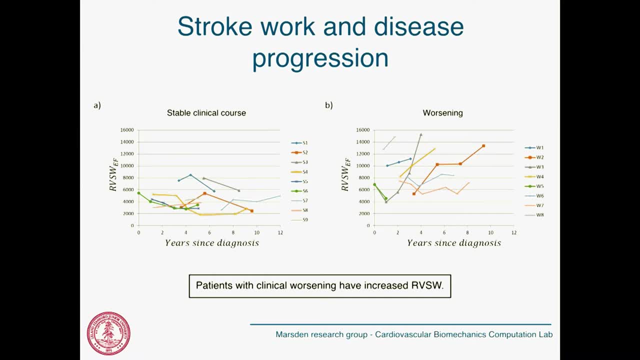 climbed quite steeply and also were on climbed quite steeply and also were, on average, quite a bit higher than in the average, quite a bit higher than in the average, quite a bit higher than in the stable group. and so we looked at stable group and so we looked at 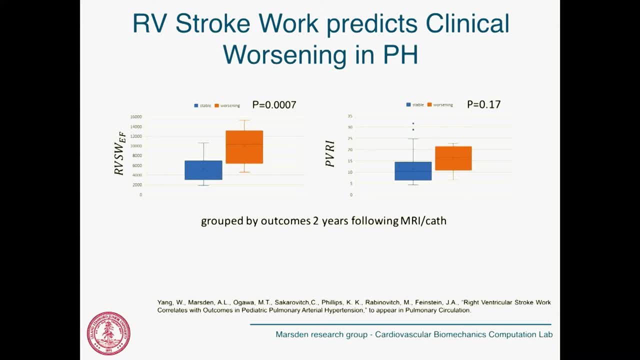 stable group, and so we looked at statistics. so we grouped for each data statistics. so we grouped for each data statistics. so we grouped for each data point in our data set. we looked at an point in our data set. we looked at an point in our data set. we looked at an outcome two years after that and then 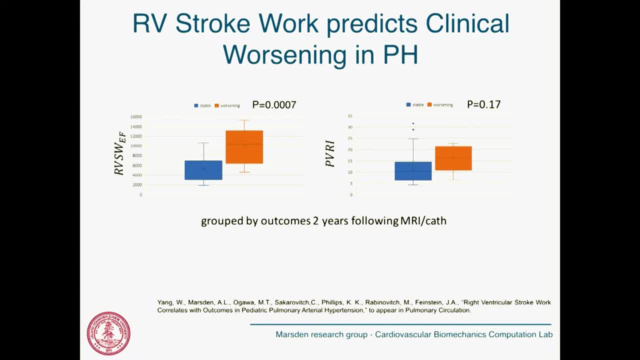 outcome two years after that, and then outcome two years after that, and then grouped those into stable and worsening, grouped those into stable and worsening, grouped those into stable and worsening, and we did show that we were able to, and we did show that we were able to, and we did show that we were able to predict clinical worsening significantly. 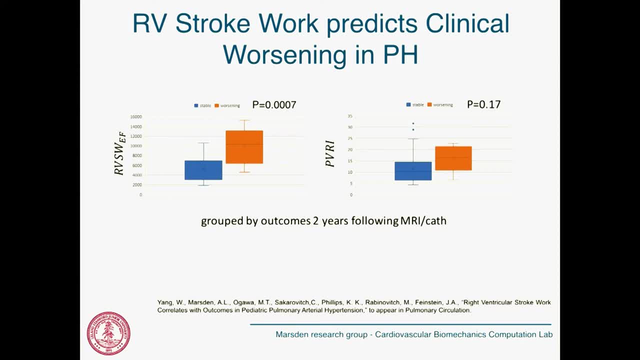 predict clinical worsening significantly. predict clinical worsening significantly using RV stroke work. and this was quite using RV stroke work and this was quite using RV stroke work and this was quite a bit better than, for example, the, a bit better than, for example, the, a bit better than, for example, the prediction value we were able to get. 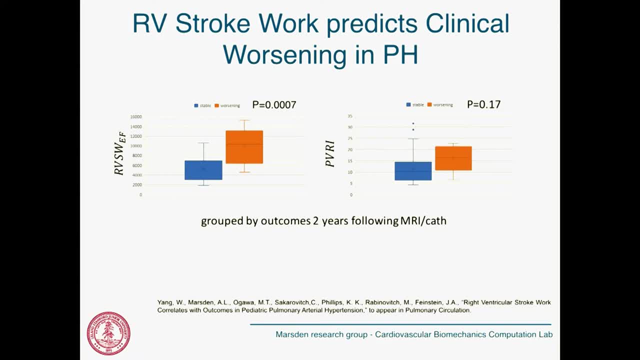 prediction value. we were able to get prediction value we were able to get with PV RI and a number of other with PV RI and a number of other with PV RI and a number of other currently used clinical metrics that we currently used clinical metrics that we currently used clinical metrics that we looked at and so we found that RV. 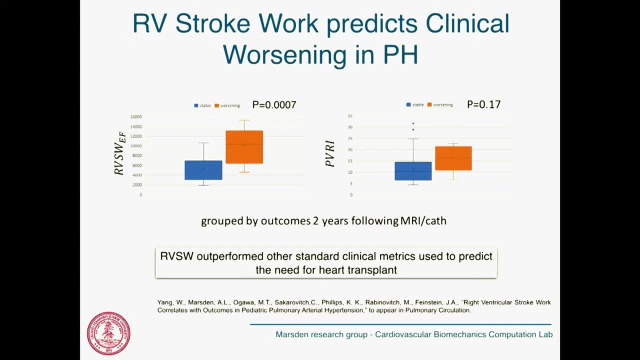 looked at, and so we found that RV looked at, and so we found that RV stroke work outperformed. other standard stroke work outperformed. other standard stroke work outperformed. other standard clinical metrics used to predict the clinical metrics used to predict the clinical metrics used to predict the need for a heart transplant. in these: 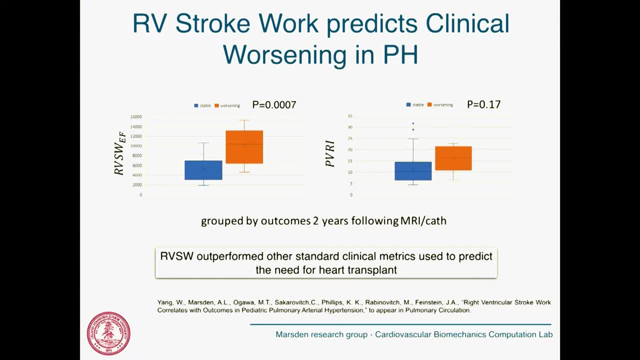 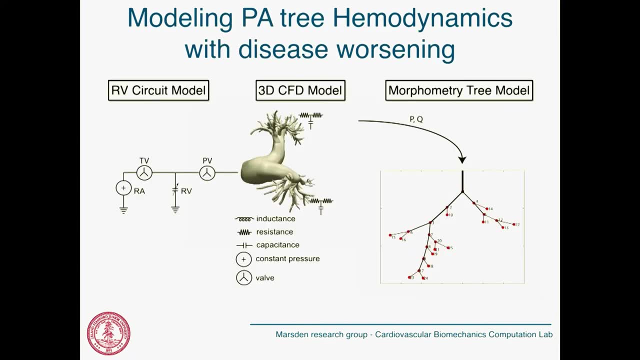 need for a heart transplant in these, need for a heart transplant in these patients, and this is just coming out patients and this is just coming out patients, and this is just coming out: soon in pulmonary circulation. okay, so soon in pulmonary circulation. okay, so soon in pulmonary circulation, okay. so getting back to our question about how, 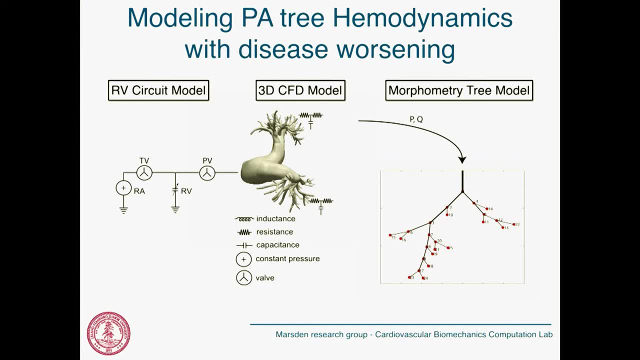 getting back to our question about how. getting back to our question about how do the hemodynamics change as you go? do the hemodynamics change as you go? do the hemodynamics change as you go down the tree and also as you progress in down the tree and also as you progress in? 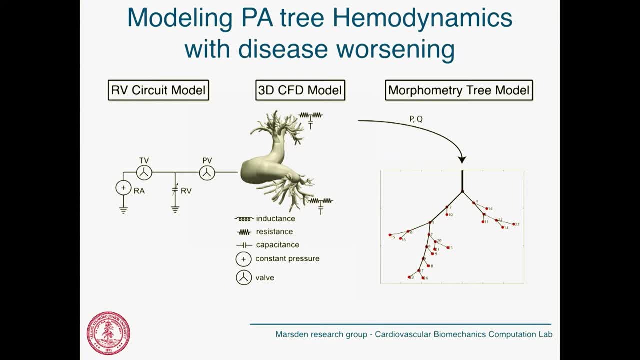 down the tree and also as you progress in terms of disease severity, in these terms of disease severity, in these terms of disease severity in these patients, and so we took our RV lump patients, and so we took our RV lump patients, and so we took our RV lump parameter model, we hooked it up to our 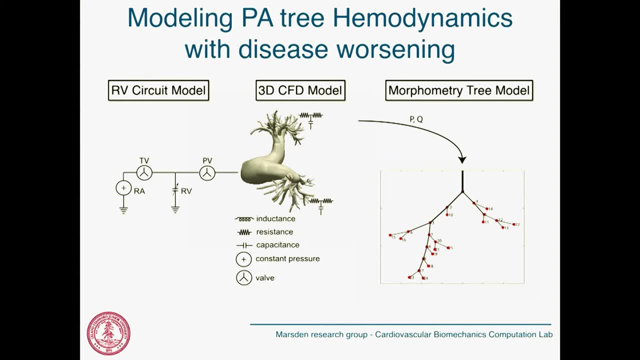 parameter model. we hooked it up to our parameter model, we hooked it up to our three-dimensional computational fluid, three-dimensional computational fluid, three-dimensional computational fluid dynamics model and then, using the same dynamics model, and then using the same dynamics model and then using the same approach that I talked about before, we 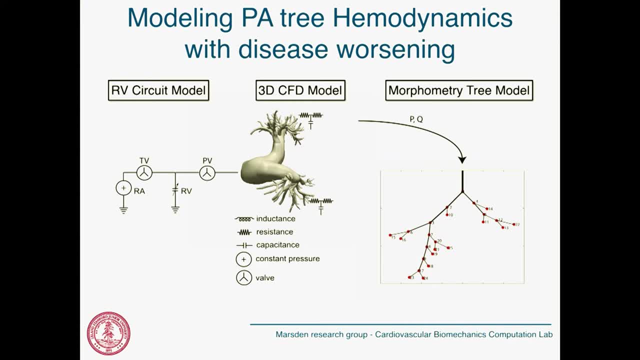 approach that I talked about before. we approach that I talked about before, we constructed morphometric trees as a constructed morphometric trees, as a constructed morphometric trees, as a separate tree, for each outlet of our separate tree, for each outlet of our separate tree, for each outlet of our three-dimensional model, to model the. 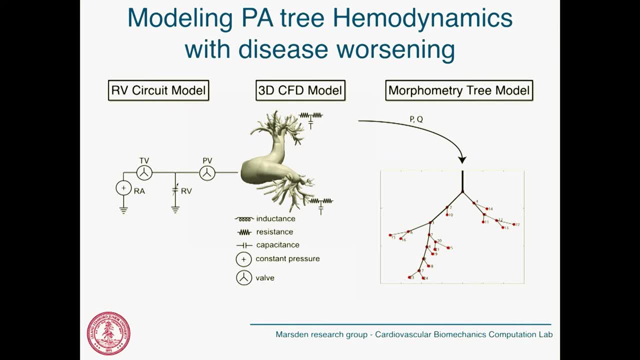 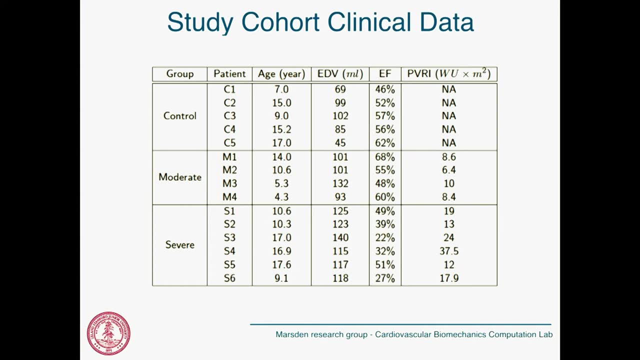 three-dimensional model to model the three-dimensional model. to model the disc distal pulmonary vasculature way. disc distal pulmonary vasculature way. disc distal pulmonary vasculature way. guang modeled five controls and then guang modeled five controls and then guang modeled five controls and then four patients with moderate pH and six. 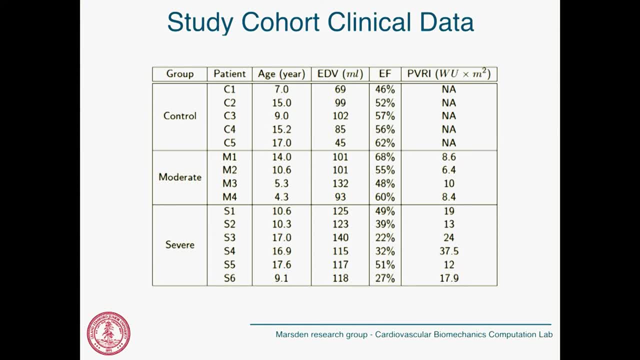 four patients with moderate pH and six. four patients with moderate pH and six patients with severe pH in the study and patients with severe pH in the study and patients with severe pH in the study and you can see their ages and some of you can see their ages and some of. 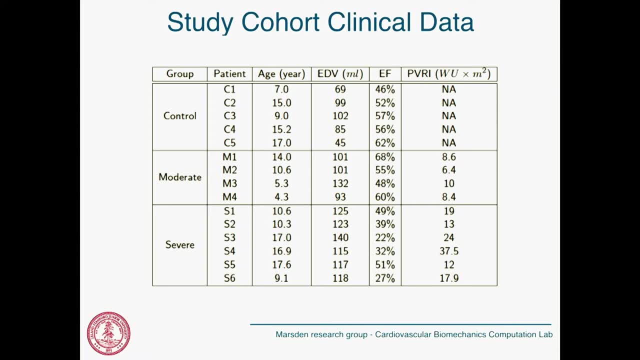 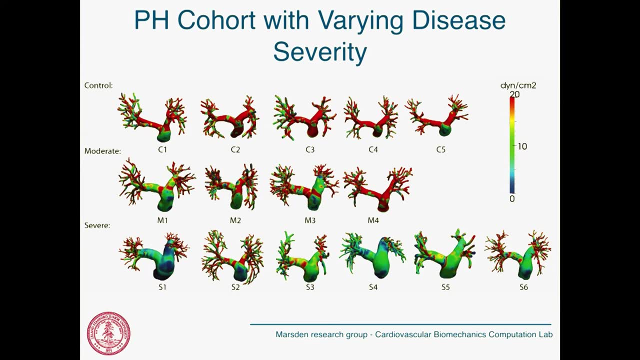 you can see their ages and some of their clinical data, like ejection fraction. their clinical data like ejection fraction. their clinical data like ejection fraction. and PV RI in this table way wrong and PV RI in this table way wrong and PV RI in this table way wrong. built three, two or three-dimensional. 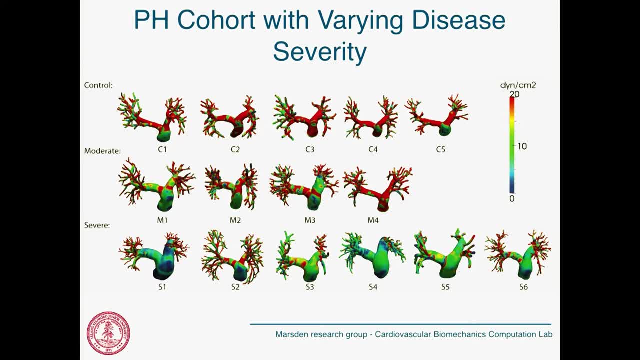 built three two or three-dimensional, built three two or three-dimensional anatomic models for all of these anatomic models, for all of these anatomic models, for all of these patients, and ran CFD simulations with patients and ran CFD simulations with patients and ran CFD simulations with fluid structure interactions. who account? 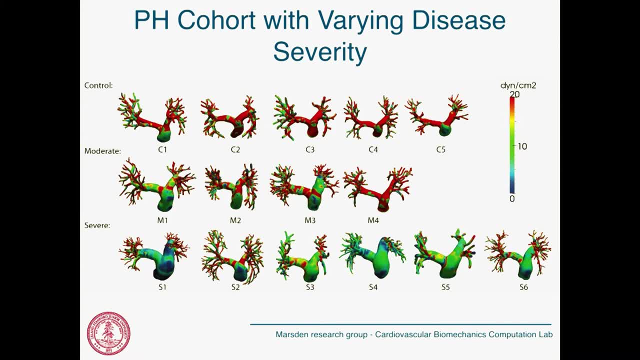 fluid structure interactions. who account? fluid structure interactions. who account for the vessel wall deformation? for all for the vessel wall deformation for all. for the vessel wall deformation, for all of the pH patients. we tuned the material of the pH patients. we tuned the material of the pH patients. we tuned the material properties of the wall to match MRI. 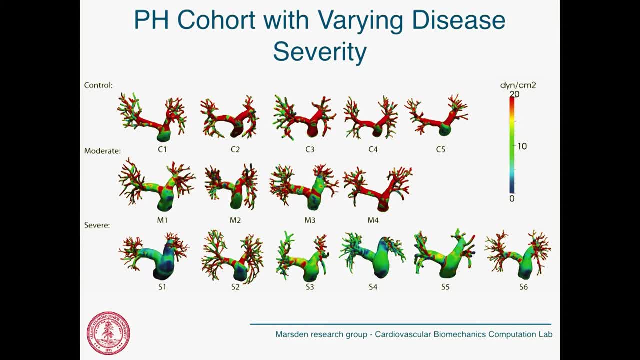 properties of the wall to match MRI. properties of the wall to match MRI derived deformation values. and so we derived deformation values, and so we derived deformation values. and so we wanted to then see both in the proximal, wanted to then see both in the proximal, wanted to then see both in the proximal PAs and in the distal PAs. how did the 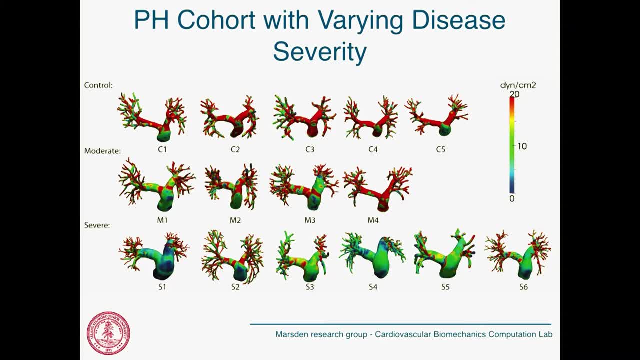 PAs and in the distal PAs. how did the PAs? and in the distal PAs, how did the human dynamics vary with disease? human dynamics vary with disease. human dynamics vary with disease: severity compared to control. so this is severity compared to control. so this is. 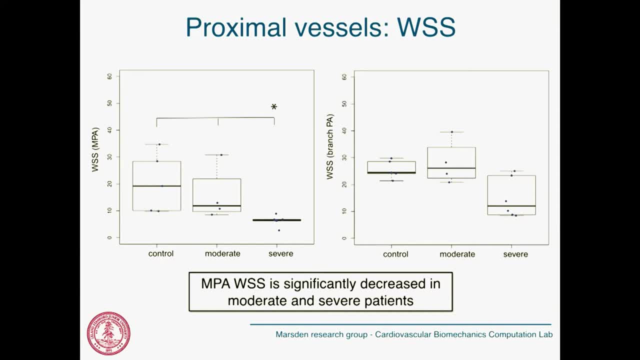 severity compared to control. so this is looking at the wall shear stress in the, looking at the wall shear stress in the, looking at the wall shear stress in the MPA, looking at the control group versus MPA, looking at the control group versus MPA, looking at the control group versus the moderate pH and the severe pH, so as 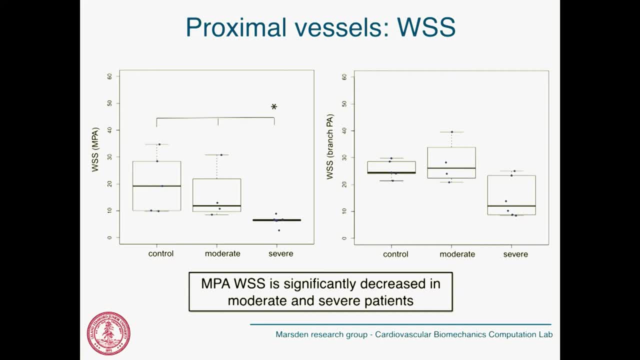 the moderate pH and the severe pH. so as the moderate pH and the severe pH. so, as expected and in agreement with the expected and in agreement with the expected and in agreement with the previous data, we do see a significant previous data. we do see a significant previous data. we do see a significant decrease in wall shear stress in the 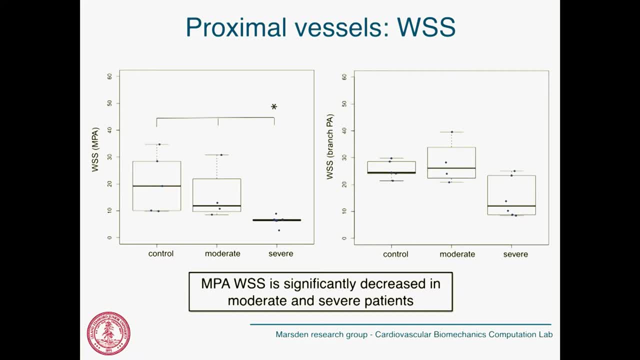 decrease in wall shear stress. in the decrease in wall shear stress in the MPA and looking at the branch PAs, we do MPA and looking at the branch PAs, we do MPA and looking at the branch PAs, we do see a decrease in the severe patient. 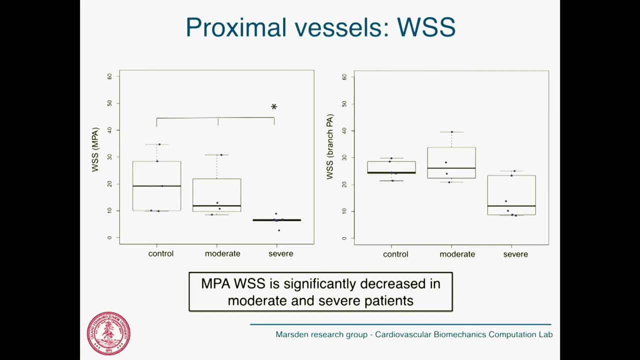 see a decrease in the severe patient, see a decrease in the severe patient group and the other two are relatively group. and the other two are relatively group and the other two are relatively similar. looking at oscillatory shear: similar. looking at oscillatory shear: similar. looking at oscillatory shear index. so this is the degree of 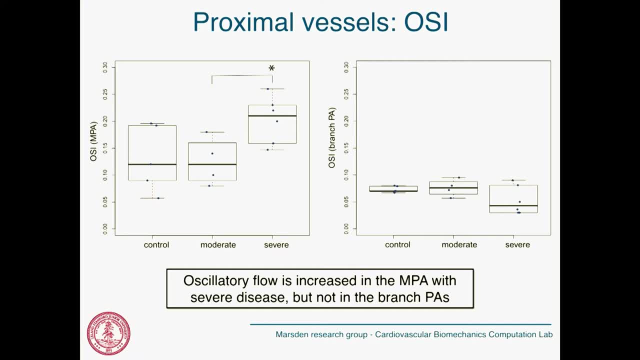 index. so this is the degree of index, so this is the degree of oscillatory flow in these vessels. we do oscillatory flow in these vessels. we do oscillatory flow in these vessels. we do see a significant increase in the MPA in see a significant increase in the MPA in. 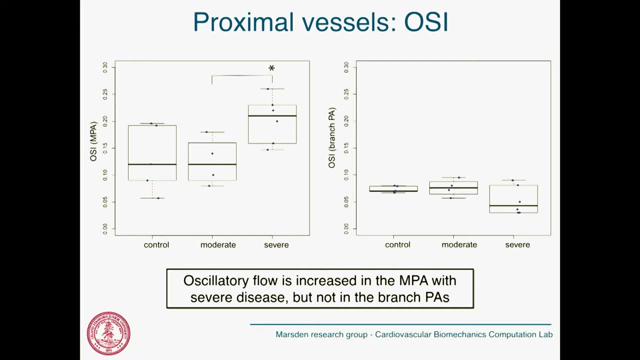 see a significant increase in the MPA in terms of oscillatory flow, in the severe terms of oscillatory flow, in the severe terms of oscillatory flow in the severe group, and little change. sorry, this keeps group and little change. sorry, this keeps group and little change. sorry, this keeps going on and off. we see, we don't see any. 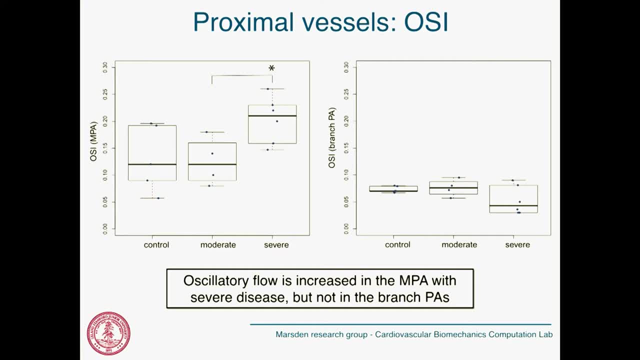 going on and off. we see we don't see any going on and off. we see we don't see any significant change in the branch PAs, in significant change in the branch PAs, in significant change in the branch PAs in terms of oscillatory flow. we also 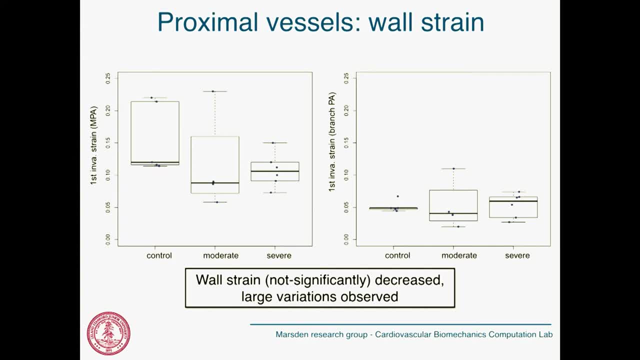 terms of oscillatory flow. we also terms of oscillatory flow. we also looked at wall strain. since we're doing looked at wall strain, since we're doing looked at wall strain, since we're doing fluid structure interaction, we could fluid structure interaction, we could fluid structure interaction. we could look at the wall deformation and we 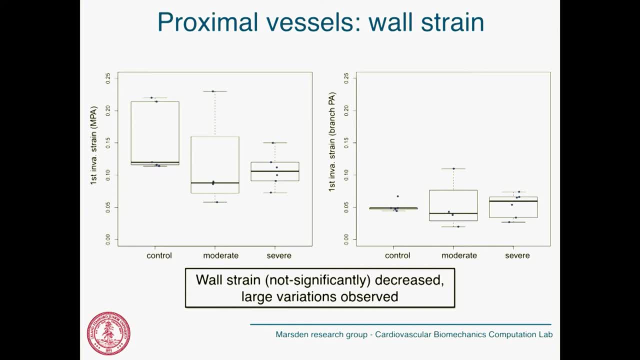 look at the wall deformation and we look at the wall deformation and we found that wall strain was decreased, found that wall strain was decreased, found that wall strain was decreased, but not with statistical significance, but not with statistical significance, but not with statistical significance, although we also saw quite a bit of. 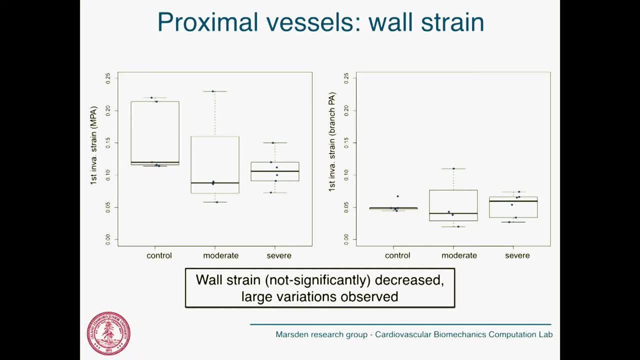 although we also saw quite a bit of. although we also saw quite a bit of variation among the different patients, in variation among the different patients, in variation among the different patients. in particular, we had an outlier who was particular. we had an outlier who was particular. we had an outlier who was very young and likely had much more. 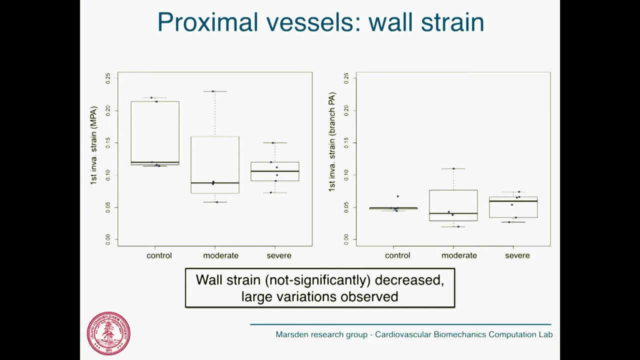 very young and likely had much more very young and likely had much more elastic vessels than the rest of the elastic vessels, than the rest of the elastic vessels, than the rest of the group. the trend overall was that we saw group. the trend overall was that we saw. 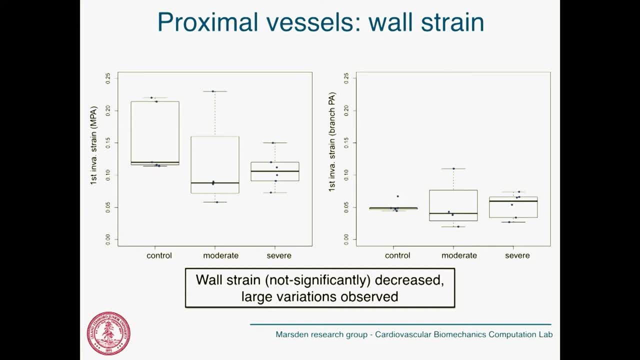 group. the trend overall was that we saw a decrease in wall strain and then an a decrease in wall strain and then an- a decrease in wall strain and then an increase, and this is really due to the increase, and this is really due to the increase and this is really due to the balance of the stiffening of the vessel. 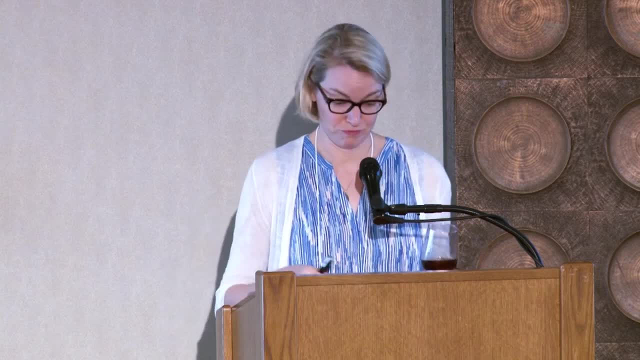 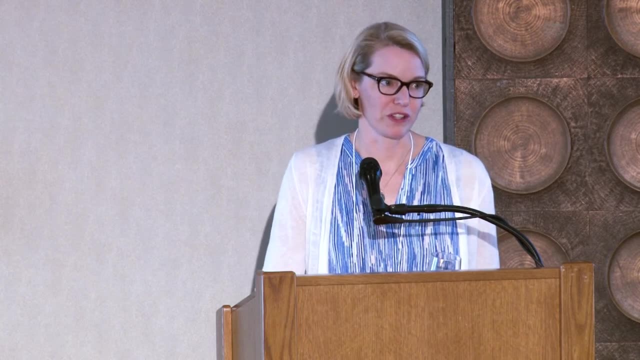 balance of the stiffening of the vessel, balance of the stiffening of the vessel walls against the increasing pulmonary walls, against the increasing pulmonary walls, against the increasing pulmonary pressure. looking at the distal vessels pressure, looking at the distal vessels pressure, looking at the distal vessels, is where things start to get really. 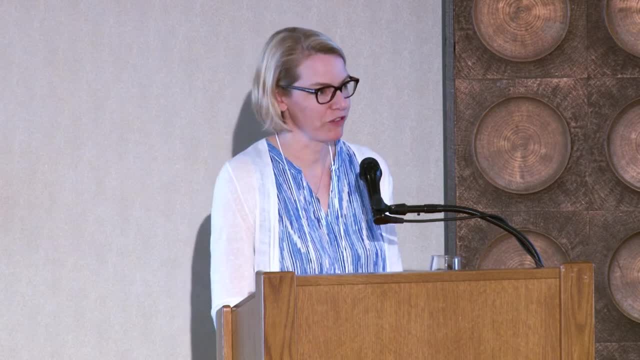 is where things start to get really, is where things start to get really interesting, because I think people have interesting, because I think people have interesting, because I think people have primarily been focused on this data, primarily been focused on this data, primarily been focused on this data that's come out showing this, the shear. 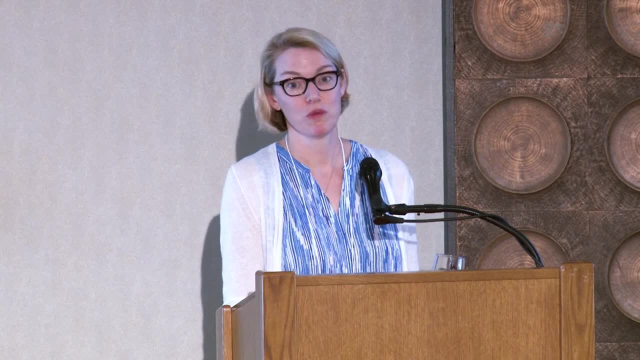 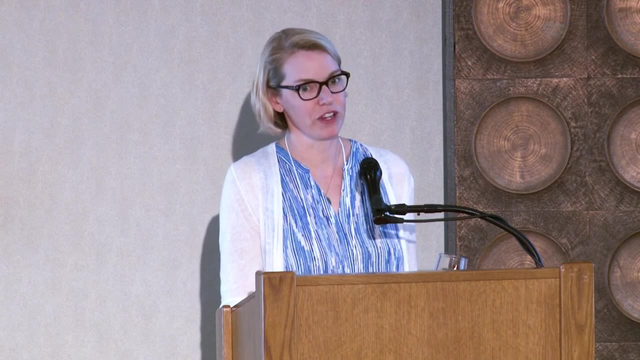 that's come out, showing this, the shear that's come out, showing this, the shear stress is decreased in the main. stress is decreased in the main. stress is decreased in the main pulmonary arteries. but what we see in pulmonary arteries, but what we see in pulmonary arteries, but what we see in shear stress in the distal pulmonary 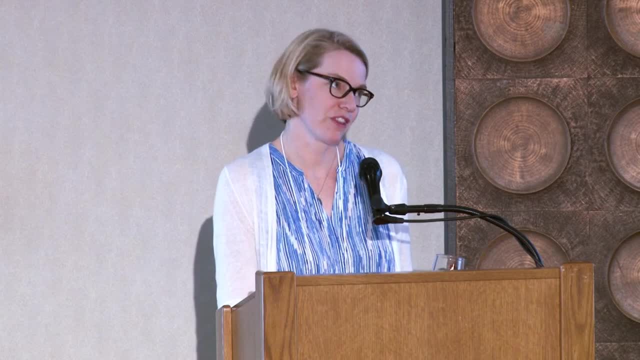 shear stress in the distal pulmonary, shear stress in the distal pulmonary vasculature, and so if we're can, if we're vasculature, and so if we're can, if we're vasculature, and so if we're can, if we're thinking about the endothelial response, 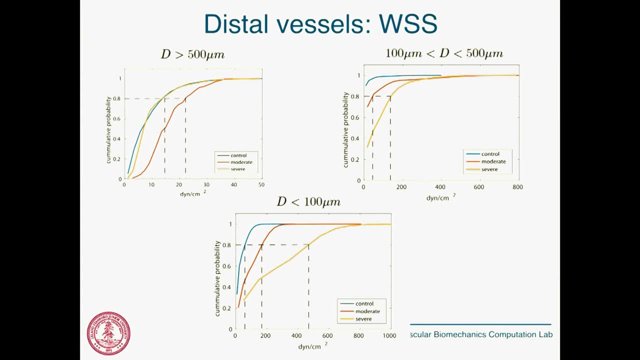 thinking about the endothelial response, thinking about the endothelial response in the PA vessels, particularly where we in the PA vessels, particularly where we in the PA vessels, particularly where we get the disease originating in the get, the disease originating in the get, the disease originating in the distal vasculature. I think what we really 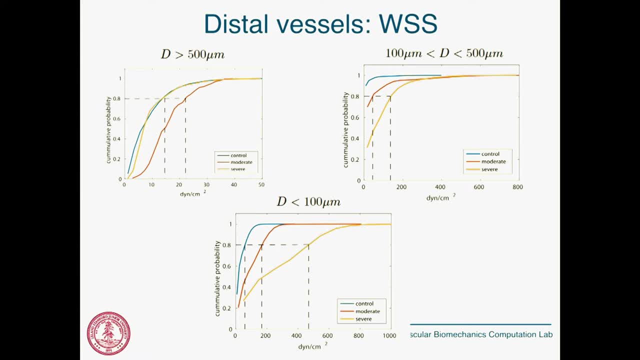 distal vasculature. I think what we really distal vasculature, I think what we really need to be looking at is is what need to be looking at is is what need to be looking at is is what happens to the endothelial cells under. 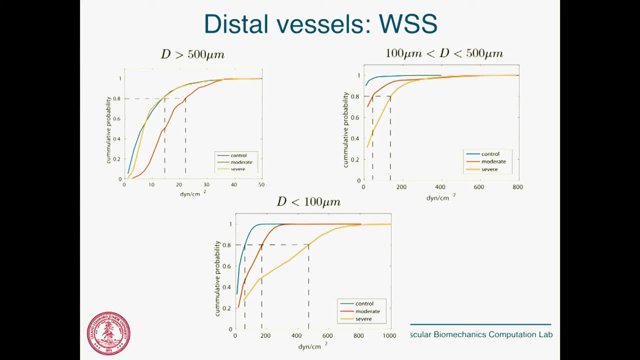 happens to the endothelial cells under happens to the endothelial cells under under severely elevated shear stress and under severely elevated shear stress and under severely elevated shear stress, and what we're seeing in our models, again by what we're seeing in our models, again by what we're seeing in our models, again by looking at the morphometric trees, and 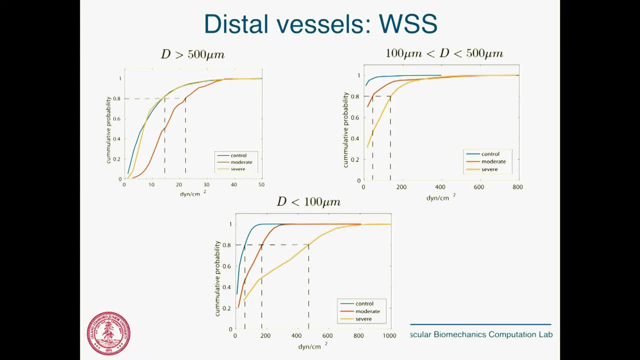 looking at the morphometric trees and looking at the morphometric trees and estimating the shear stress at different estimating the shear stress at different. estimating the shear stress at different sized vessels. is we're seeing values sized vessels? is we're seeing values sized vessels? is we're seeing values upwards of a hundred in the say two, three? 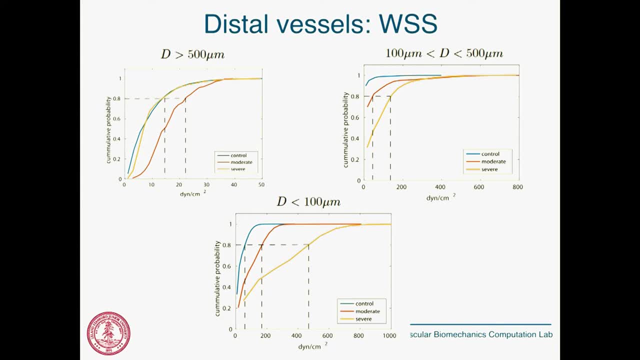 upwards of a hundred in the say two, three, upwards of a hundred in the say two, three, four hundred range. and these are four hundred range and these are values that have not been previously looked at experimentally in the context of pH, and so we're now collaborating with Marlene's group to start doing some. 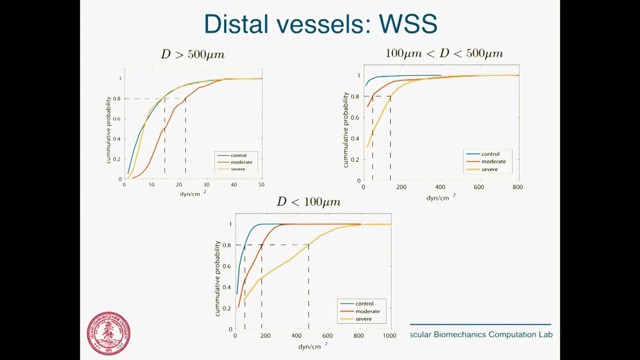 experiments, and they've already got some, some interesting data along these lines, and so, again, just what you're seeing here is these are cumulative distribution plots, so what you're seeing is a probability that a vessel in this size size range will have a shear stress of this value. so, for example, 80%. 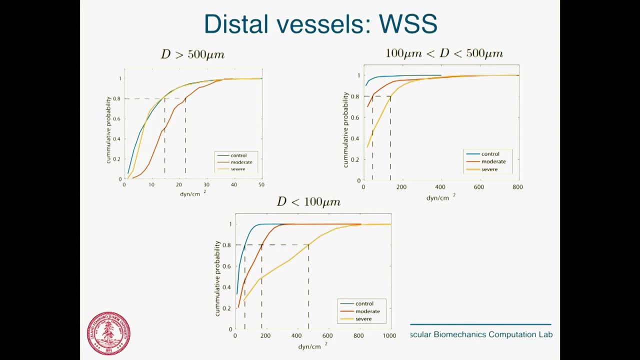 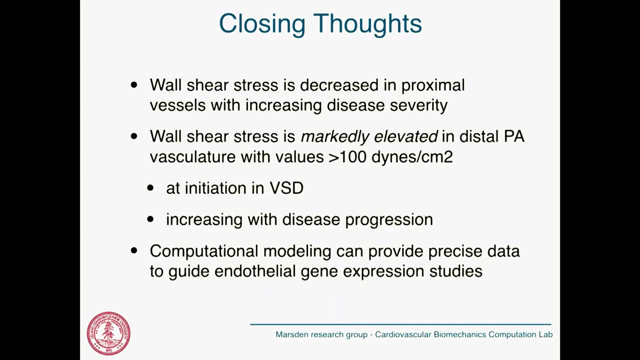 probability that the vessels in the moderate group will have a shear stress of 20 over. here you can see we're really getting severely elevated values, especially in the severe group in the- you know- several hundred dynes per centimeter squared range. so just to close, I think our data is in agreement with prior data that while 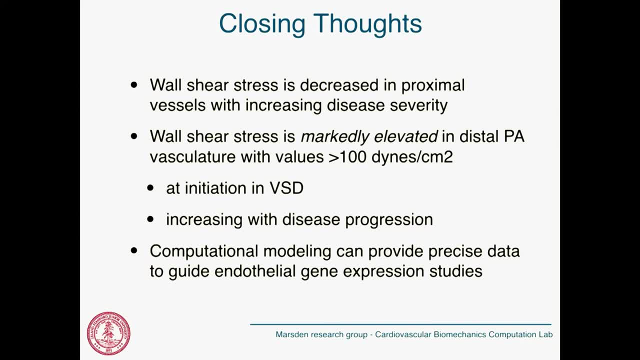 shear stress is decreased in the proximal vessels with increasing disease severity, but we believe it's markedly elevated in the distal PA vasculature, with values upwards of a hundred dynes per centimeter squared, and this is likely has implications for initiation of pH, for example in patients with. 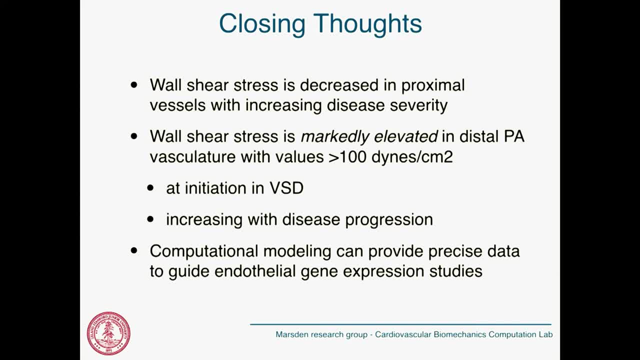 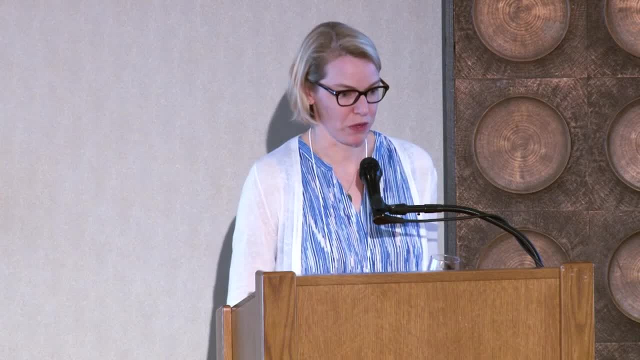 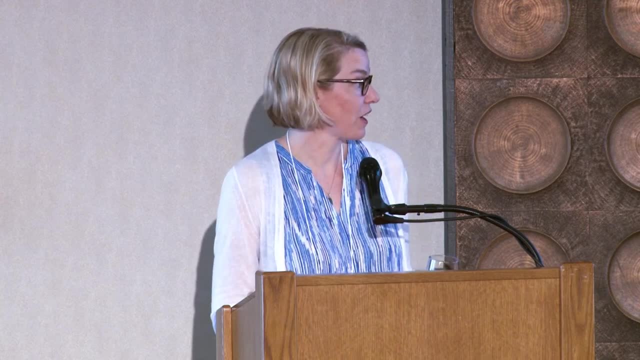 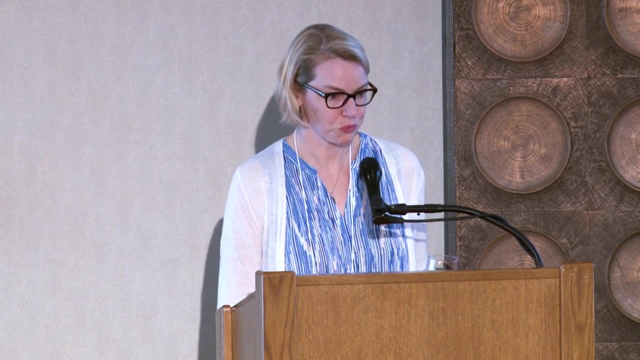 congenital heart disease, and then we see these values increasing even more with disease severity when we look at patients with progressively worsening pH. so we believe that computational modeling can provide more precise data to guide sort of what are the targeted endothelial gene expression studies that we should be looking at. I'll just close by saying that I think 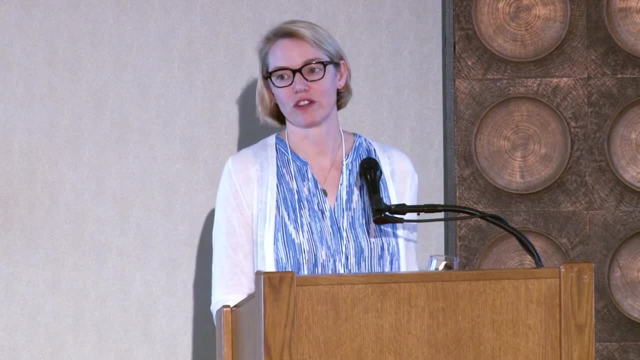 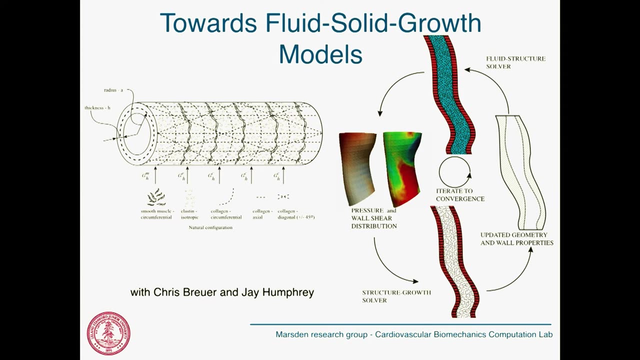 another direction that we're going in is to start looking at vascular growth and remodeling and how we can incorporate those processes directly into our computational models. so what? we're collaborating with Jay Humphrey at Yale to try to merge some of these tools together, and the vision that we have is that we can eventually do a CFD study. 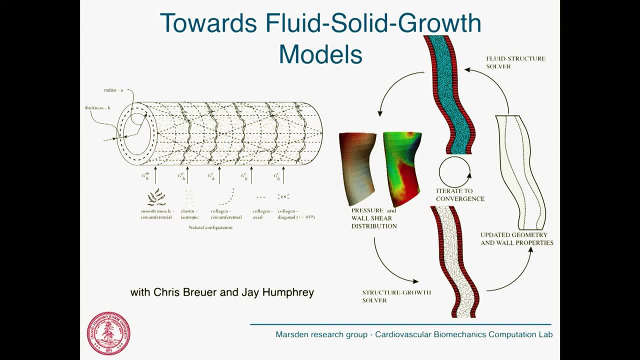 that gives us pressure and wall shear stress distribution. pass that to a structured growth solver where we can grow the vessel wall in response to those stresses right in the model. give that updated geometry back to the solver and loop through this process of altered flow conditions vessel wall. 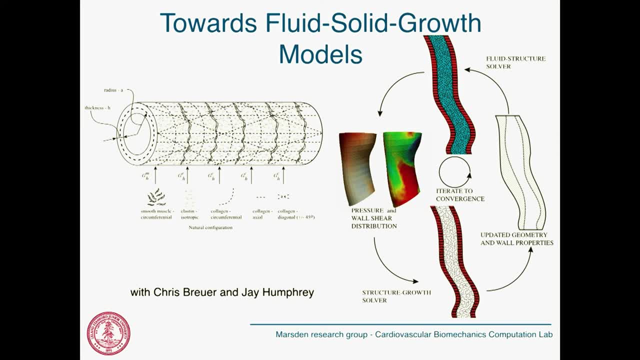 growth, increasingly altered flow conditions, etc. and so I'm very interested in applying some of those tools to the context in the context of this disease. we also have an open source project, so all of the modeling capabilities and tools that I've talked about are available to you at the Yale University School of Medicine. 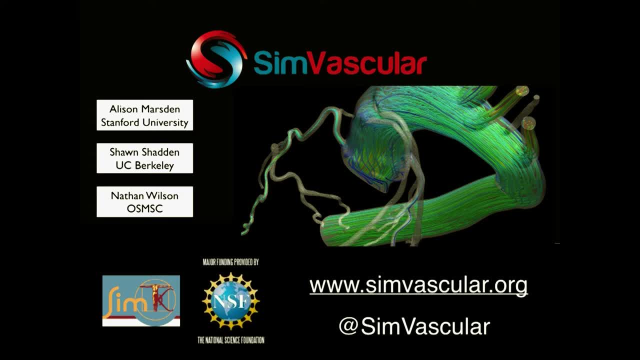 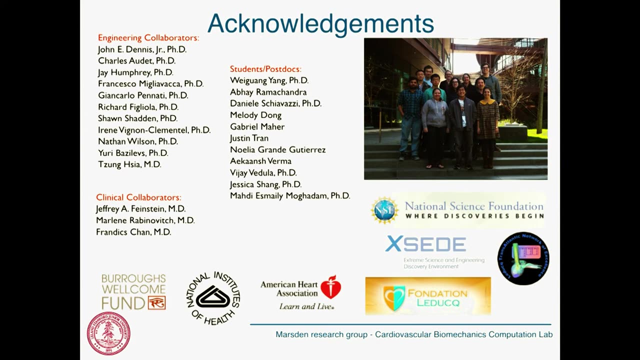 Thank you. We continue to rely on the information available at Symvascularorg for other research groups and we would love other people to use them and contribute to them, and I will just end by acknowledging particularly Melody and Weigwang, who are sitting in the back, as 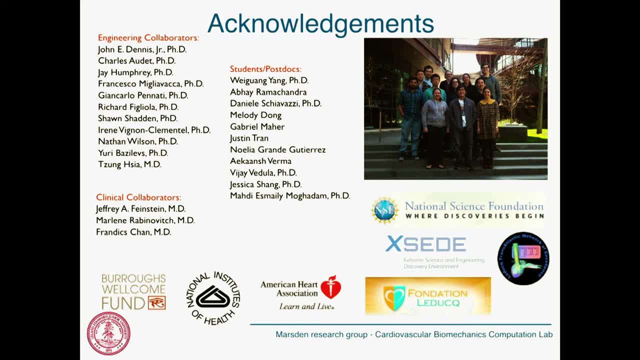 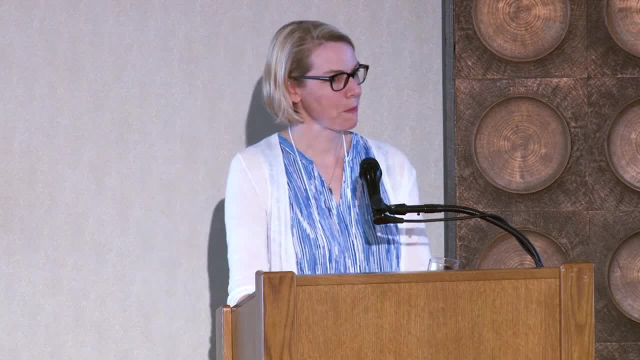 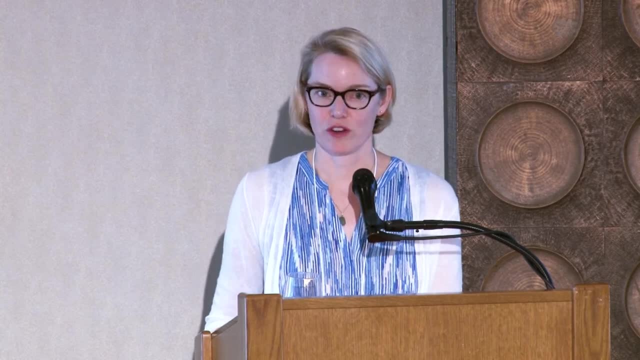 well as Jeff Feinstein, Marlene Rabinovich and Frandix Chan, who were involved in the clinical side of this project. Thanks, Happy to take questions. So the in terms of resolution of the simulation they're quite well resolved and we usually do a mesh convergence study so we end up with finite element meshes. 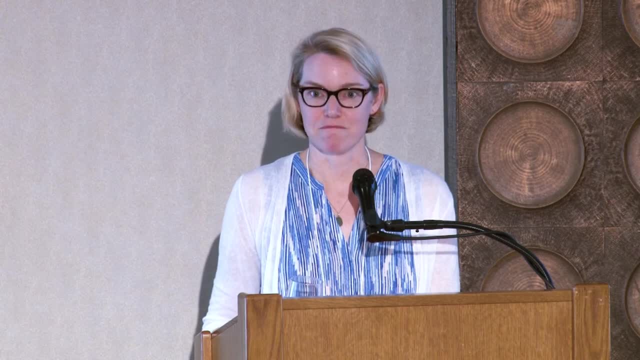 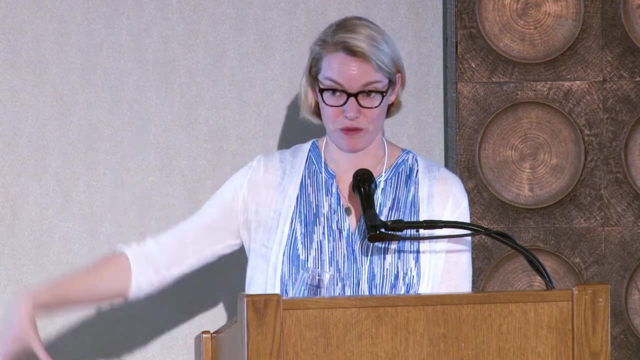 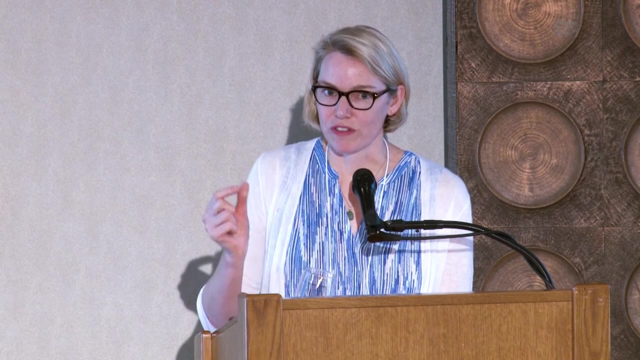 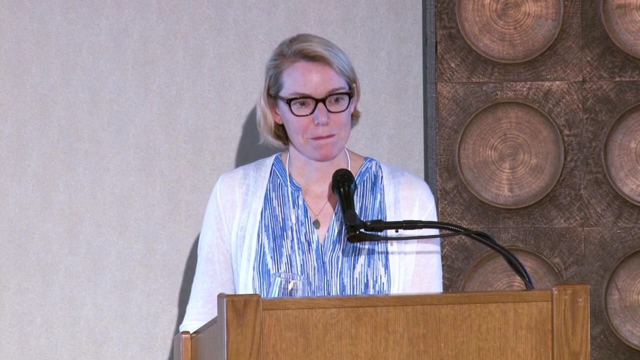 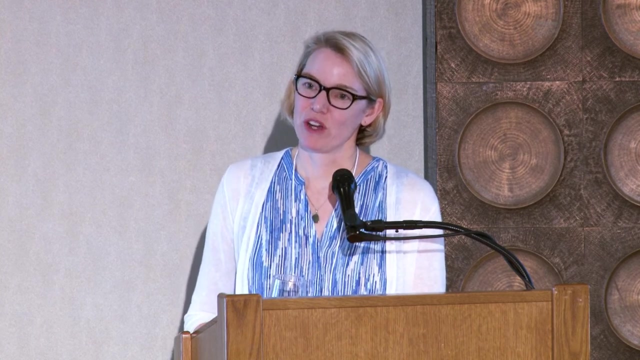 with usually several million elements. I don't remember exactly their size, but essentially we get a, you know, three components of both velocity and pressure throughout the model. in terms of the vessel, I mean, we're solving a continuum equation. so I'm I'm not sure that. I think the question is more whether the 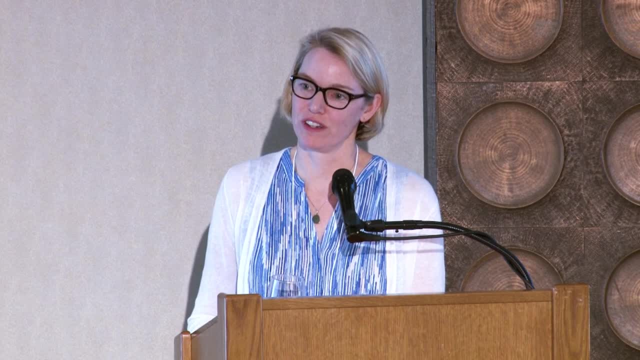 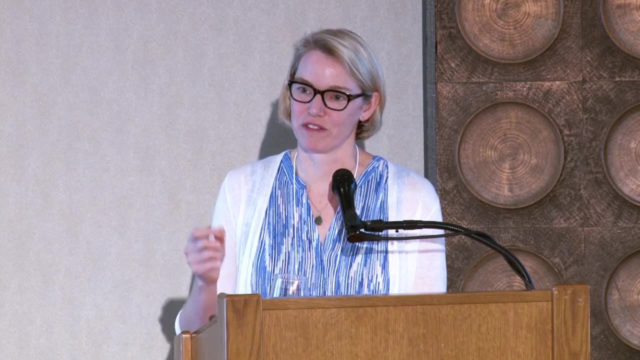 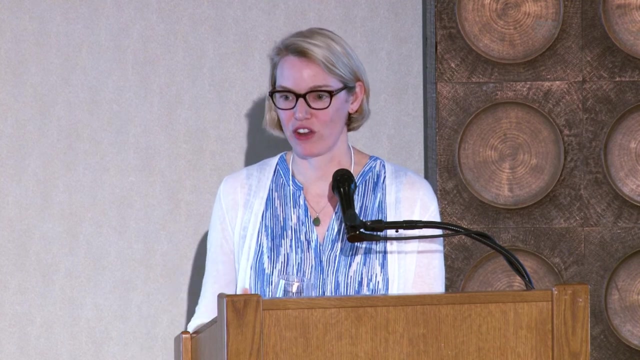 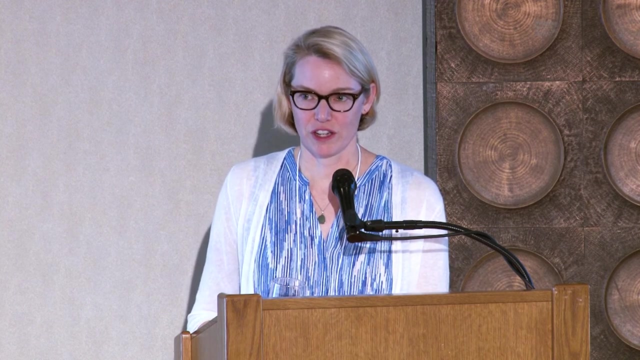 simulation is resolved, than really what the resolution is. I wouldn't say we can. I mean it depends on the question you're trying to answer in terms of how fine you want like cellular response at the vessel wall. but they are, they are converged. that that we've done, usually a couple of hours to days of compute time. 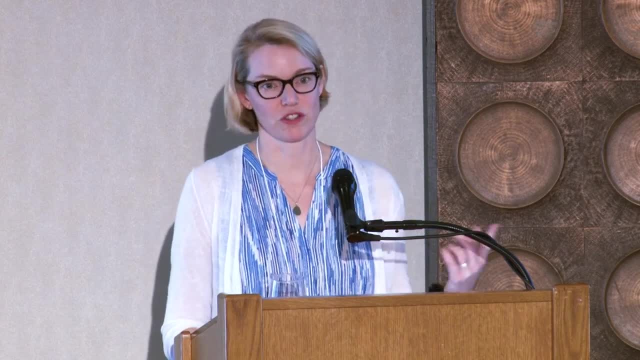 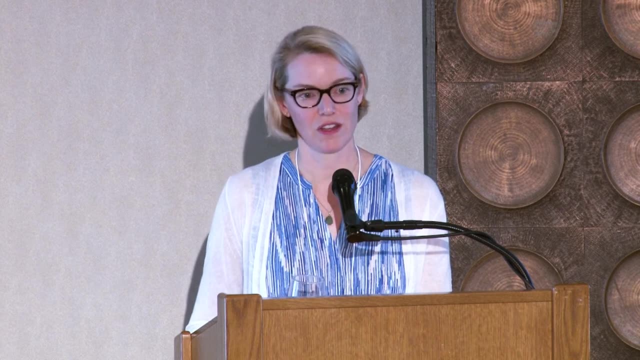 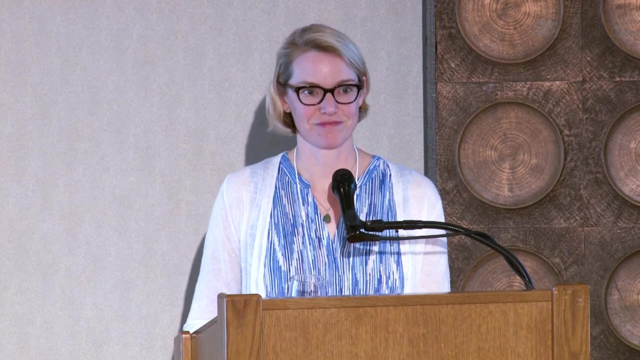 so we run these on both a local cluster here at Stanford, as well as exceed cluster, one of the next national supercomputing centers. so it usually takes- I don't know- 10 hours on multiple cores. Allison, really well done is, is the goal eventually for you to be. 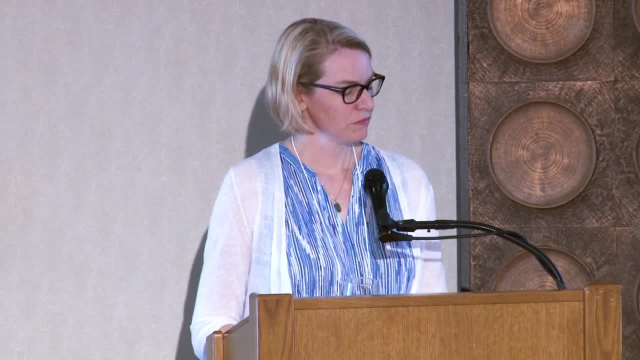 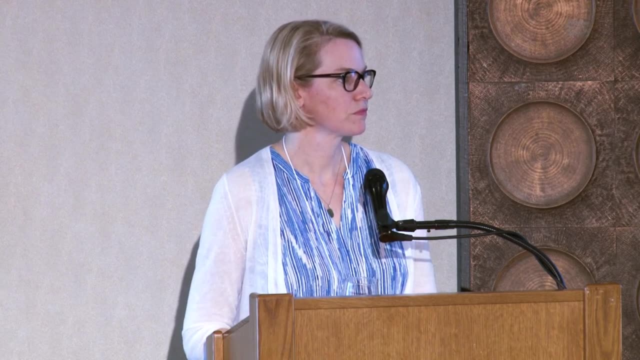 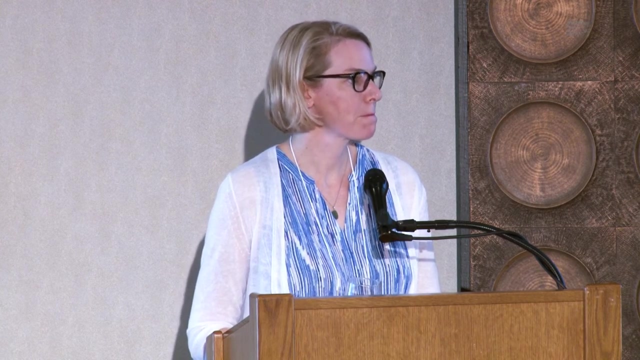 able to look at treatment response. so, for example, is the model dynamic enough that you could take a vasoreactive idiopathic patient who, on 30 seconds of nitric oxide, will substantially reduce the rate of the treatment response and reduce their PVR and improve the pulmonary compliance, and maybe study them and then 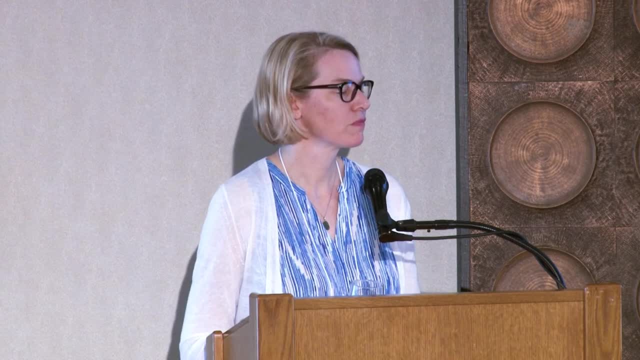 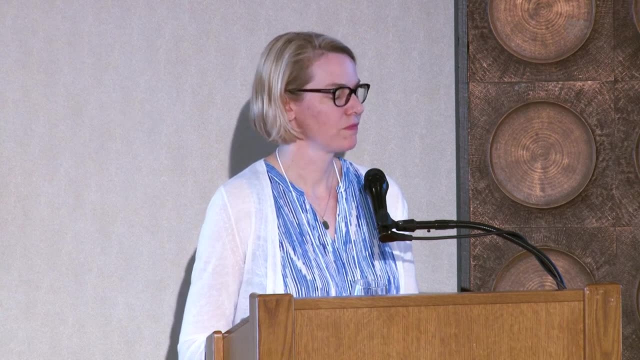 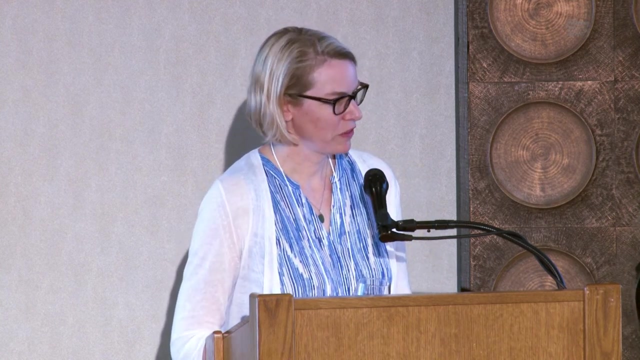 model- what a superb response would be- and then either use it as a predictive or a supportive model to decide on therapy. I wonder if you can speculate on that a little bit. so I guess the direction we've started out going is is more from the point of view of: could we predict? 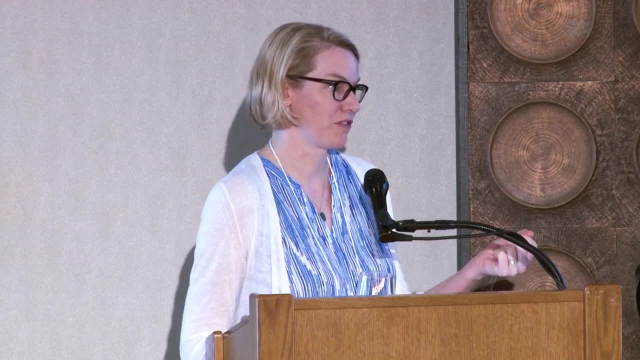 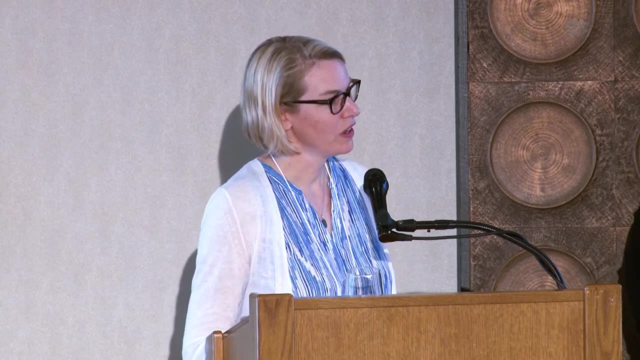 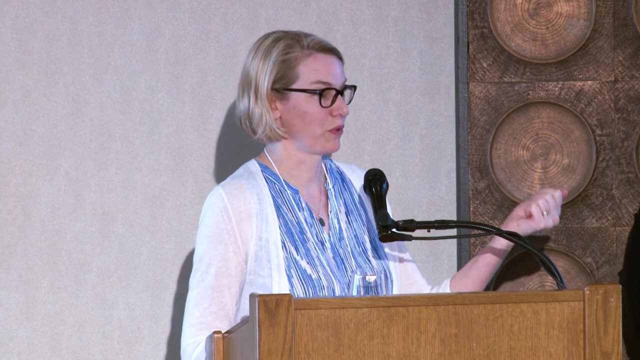 disease progression and also could we understand exactly what forces the vessel walls are experiencing. but I do think we could simulate the type of scenario that you're talking about, but the challenge there is really: you know how a pharmacological treatment would affect something like PVR. so we can. we. 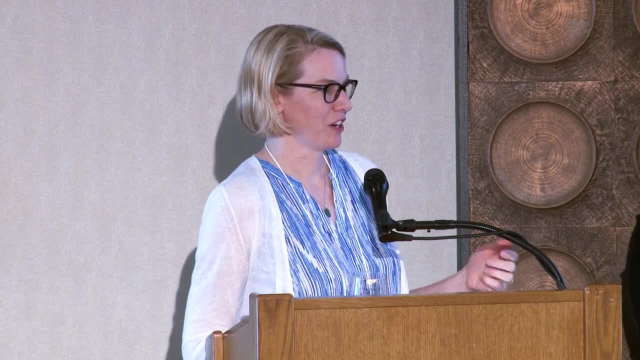 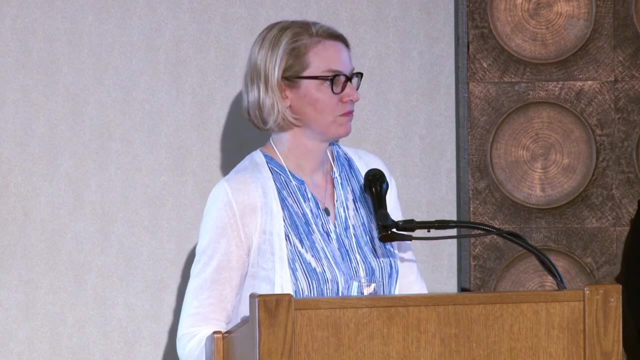 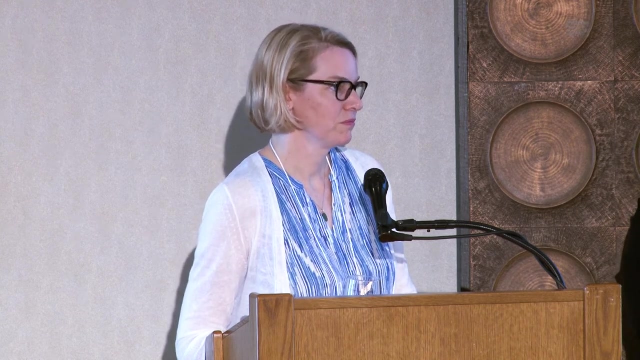 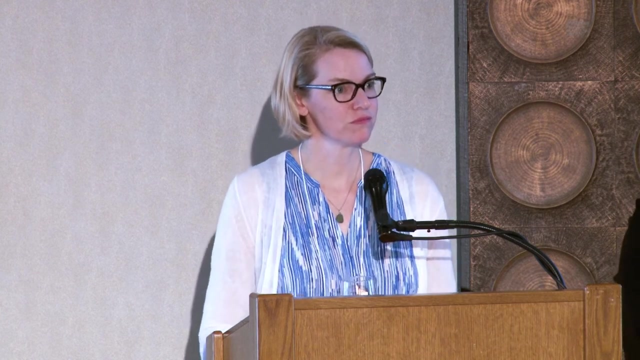 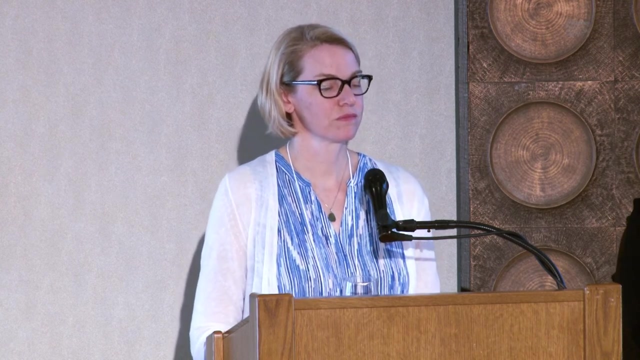 can change PVR at will in the model and then simulate the resulting conditions. yeah, so that is something I think we could do and would be interesting. so I'm a pediatric cardiologist and I'm curious: what do you think about the treat and repair strategy in the patients with borderline PVR, because I always mean a 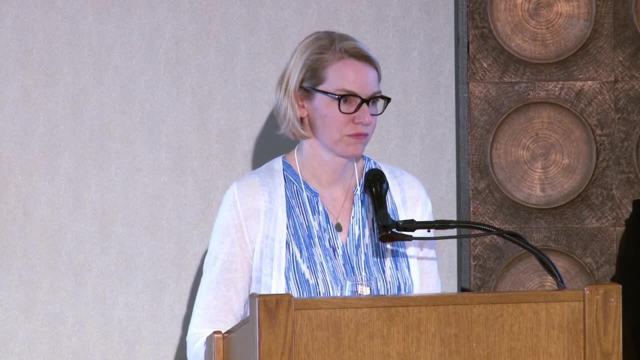 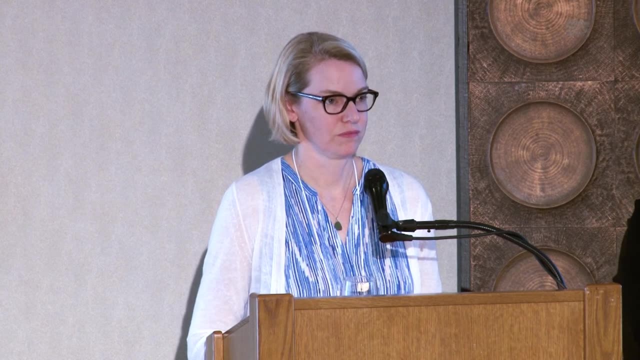 lot of people do it, but I sometimes feel you know you're giving a vasodilator to someone with an open shunt and you probably increase the flow to the pulmonary vascular tree, possibly decreasing pressure, but increasing flow. what happens to the shear stress in such 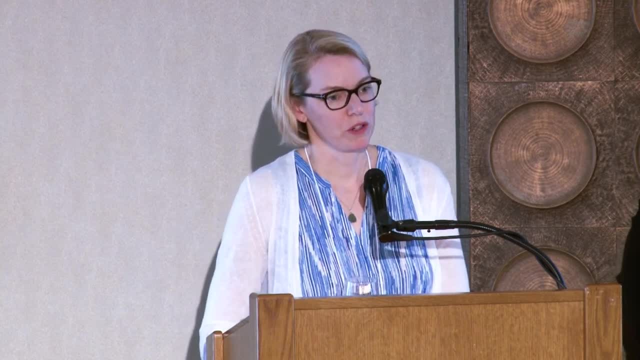 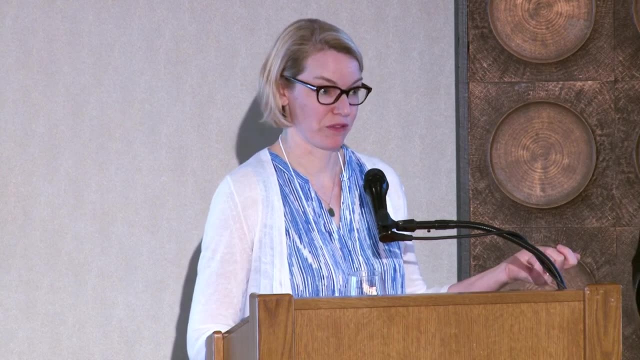 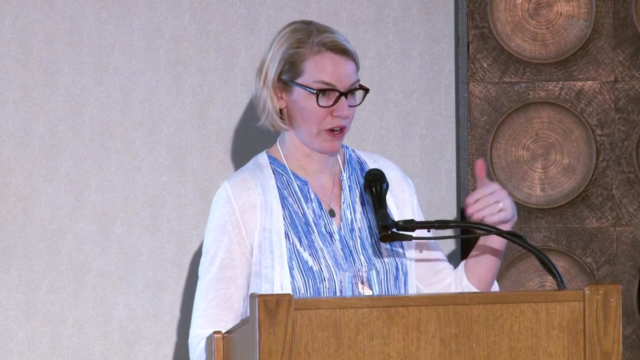 a situation, yeah. so I mean you're gonna increase. anytime you're increasing flow, you're gonna correspondingly increase shear stress and then you're gonna drive a response in the vessel wall, so exactly, and that response is going to vary depending where you are in the tree. so in 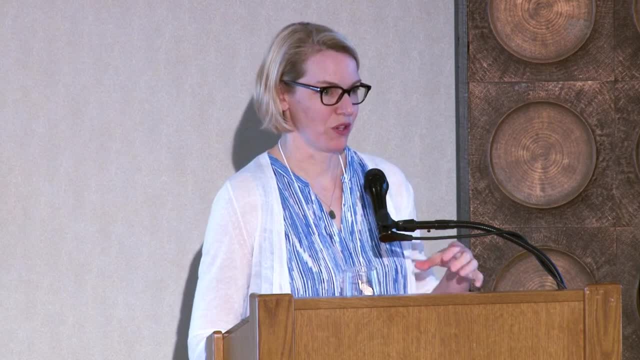 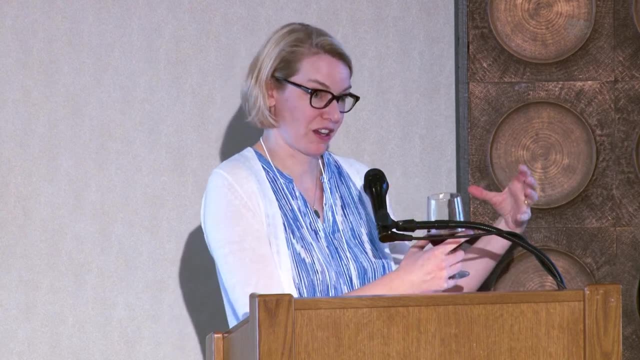 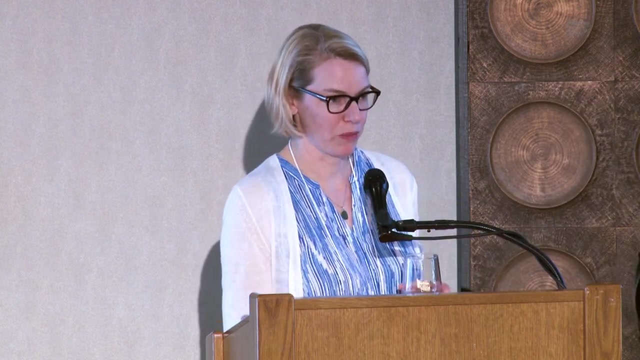 the proximal tree. you know you may get at least so, for example, with increasing pressure you're gonna. you would expect this kind of dilation in the in the proximal vessels and constriction in the distal vessels that we see in pH patients. so we would have to kind of tease out what would be the expected. 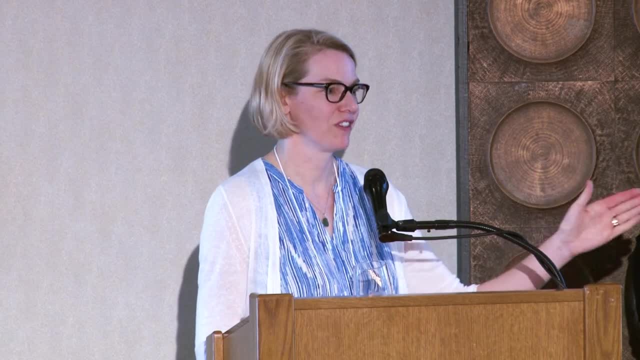 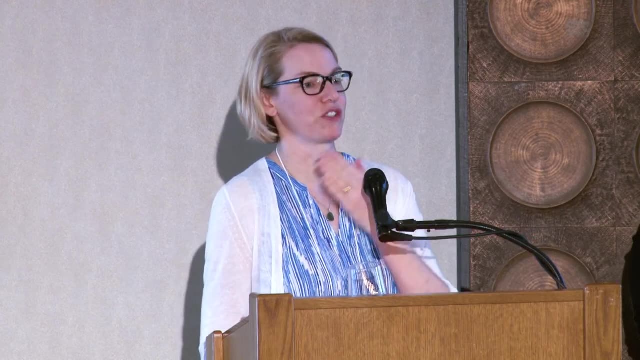 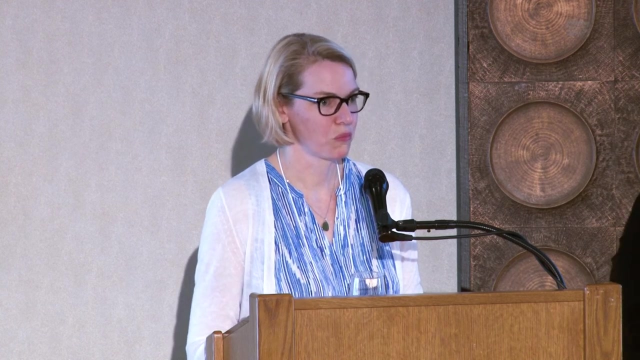 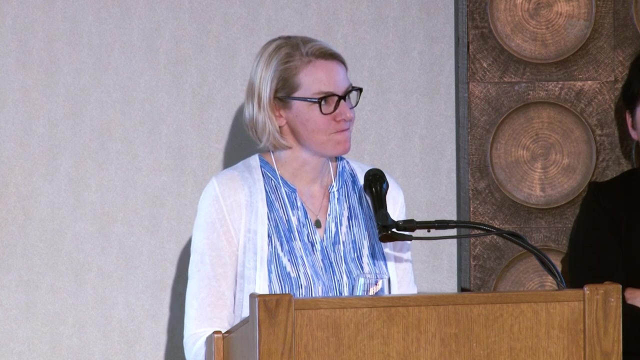 remodeling response in, so you can think about conditions where you're just increasing flow, or you're increasing both flow and pressure, or you're just increasing pressure, but and if you manage to decrease pressure and increase flow, would that be good or bad? I'm not sure we're. 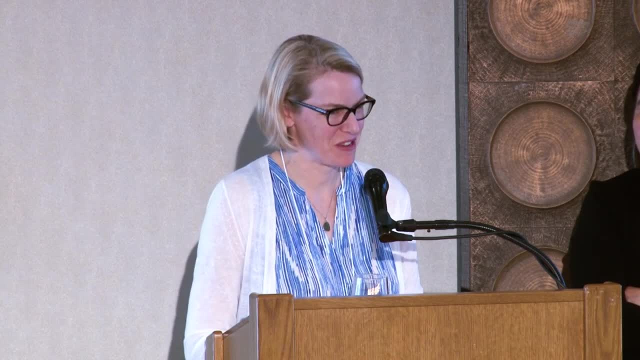 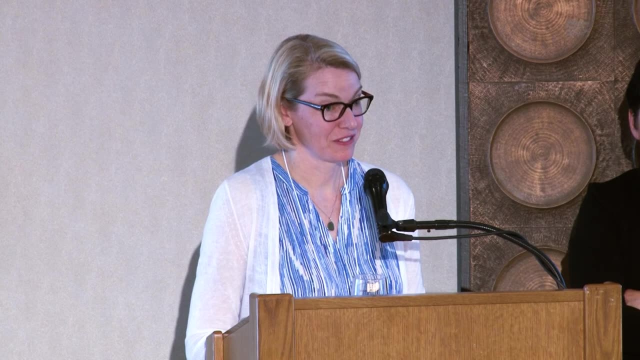 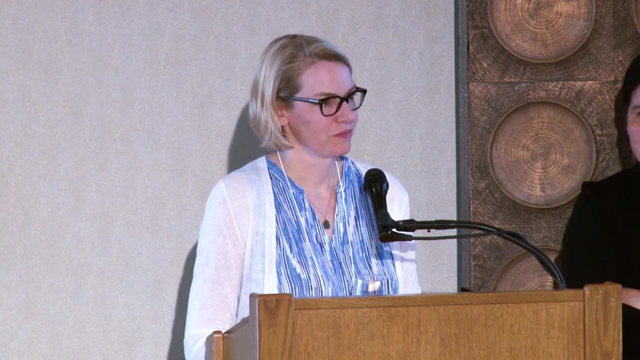 far enough along in the growth and remodeling sort of pipeline to definitively answer that question. people who are are young for treat and repair. yeah, it might be better to increase, well and decrease pressure, mm-hmm. so that's beautiful work. I have a question. that's a little bit off. 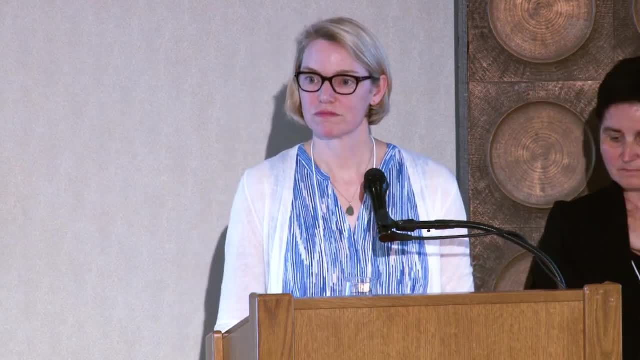 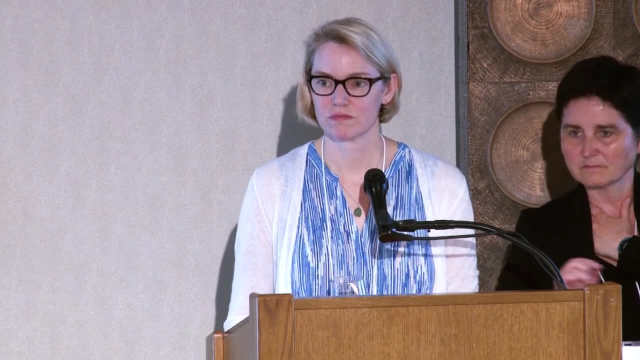 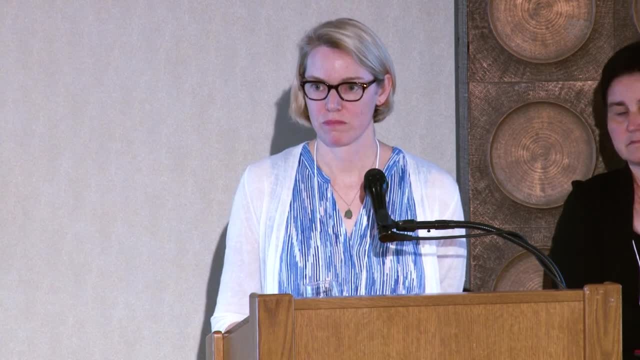 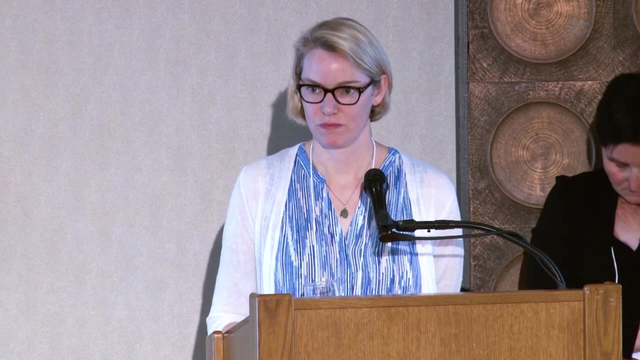 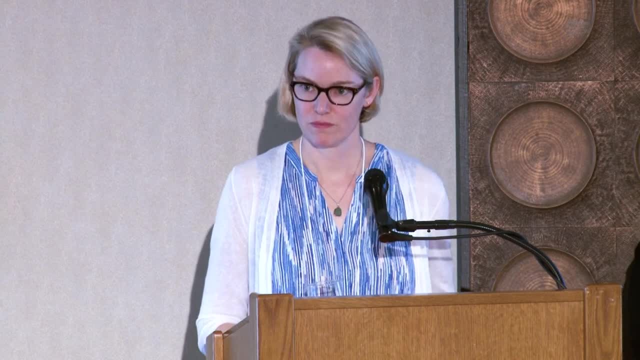 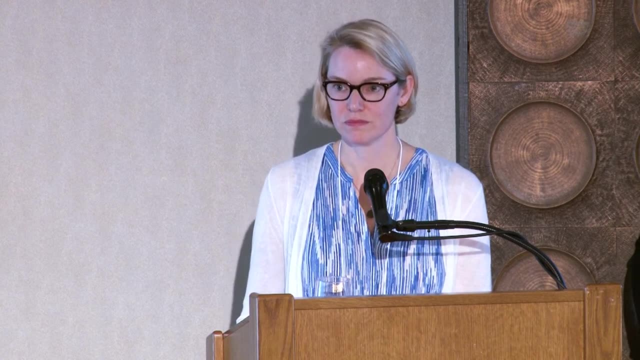 across the pulmonary circulation in PAH compared with controls and you know, as you, as you show the, the older data is suggesting that there's low shear stress. until you know, you showed your new data. we didn't have an explanation for that, but the inference is that there might. 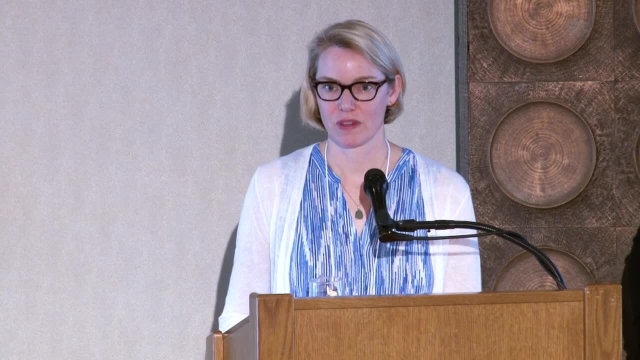 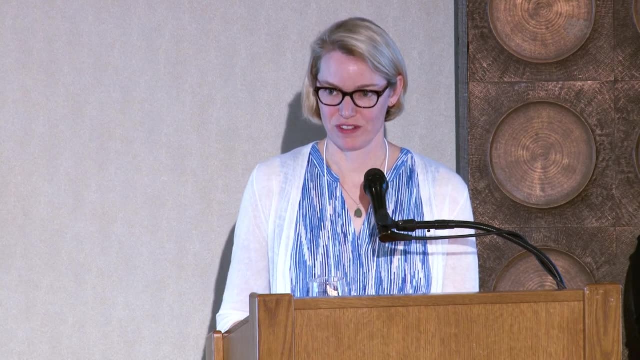 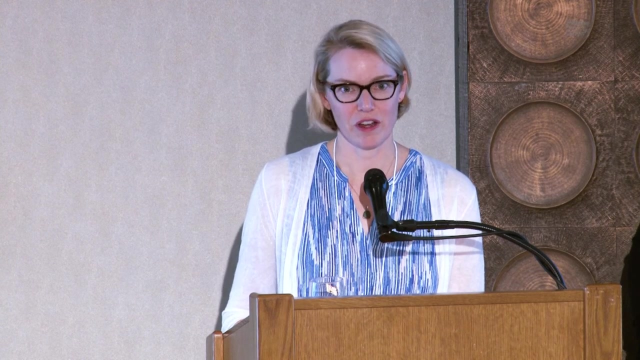 be some low-level lysis across the circulation. yeah, so I mean, we were definitely quite surprised by how high the shear stress values are, and so it would not surprise me greatly if there are in the range that could cause lysis we'd have to. I don't know. 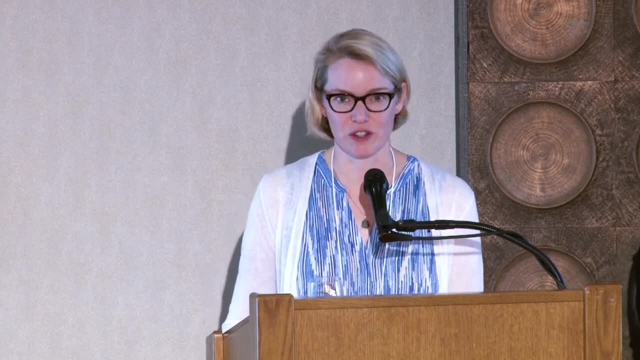 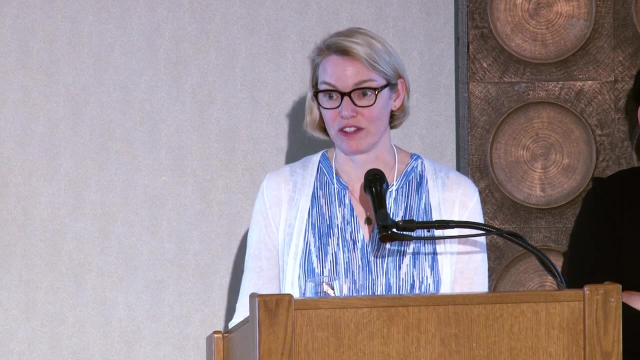 if wei guang, if you've computed strain rates we'd have, we could look at strain rates in those vessels and see, you know, if they're in that range. but yeah, we mean they're high enough that we were quite surprised by that. but yeah, we, I mean they're high enough that we were quite surprised by that. but 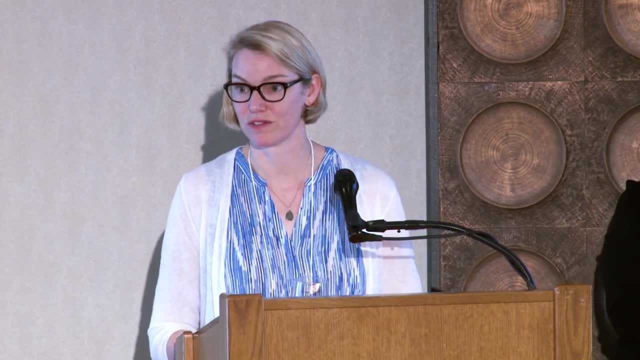 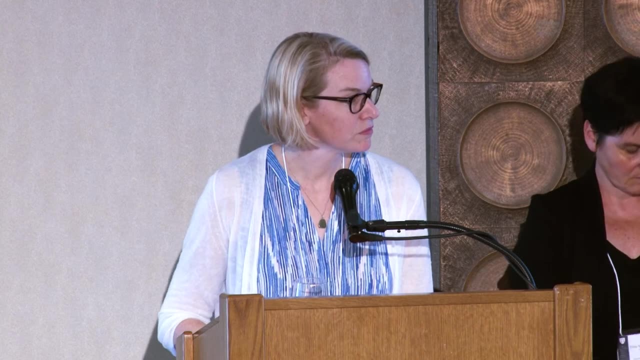 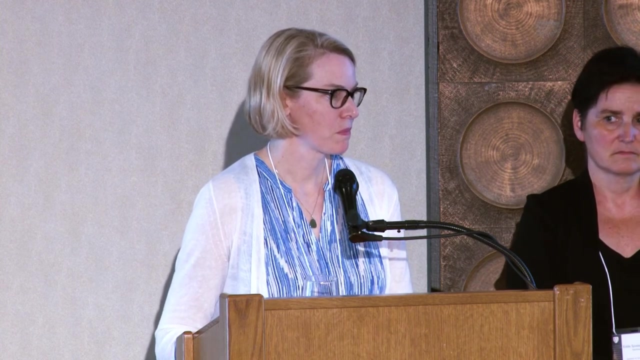 by how? just how high? all right, and I might have missed something, but I'm trying to wrap my head around why the shear stress is so high in the distal vessels, and you might have already shown this, but was this a consistent phenomenon to a similar degree both in the less severe pH? 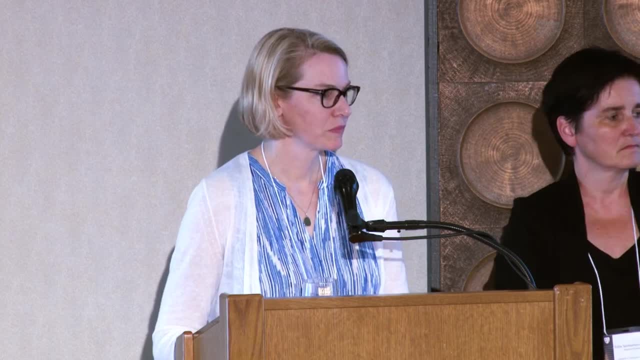 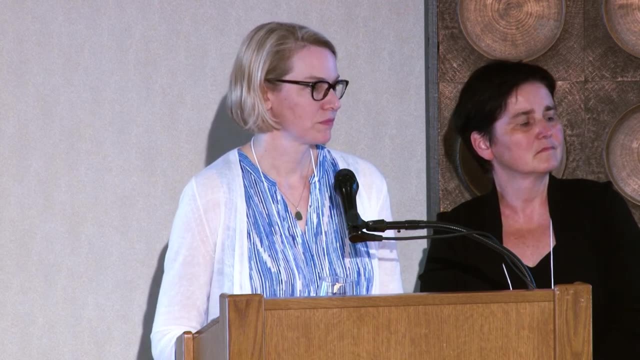 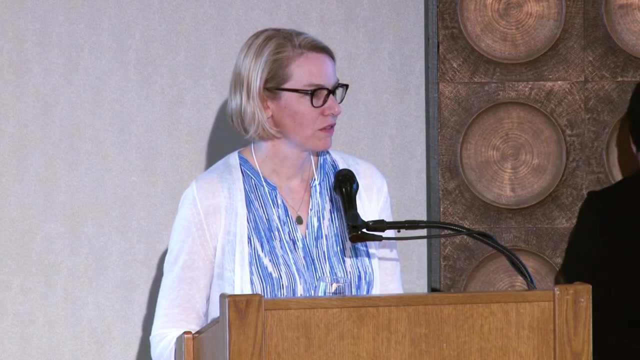 and the severe pH? and if so, is it safe to presume that the patients with severe pH had severe pruning? so why would that effect be similar? You'd think you'd see less of a rise in distal shear stress in the less severe, less pruned. 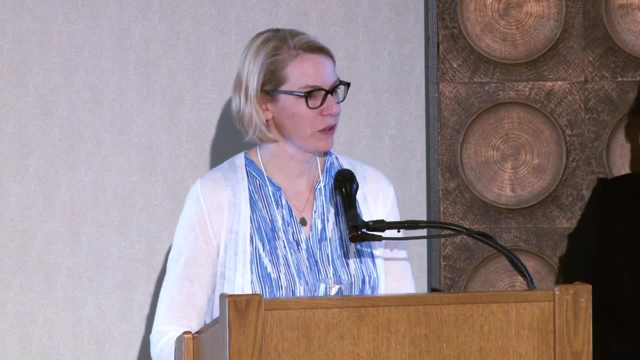 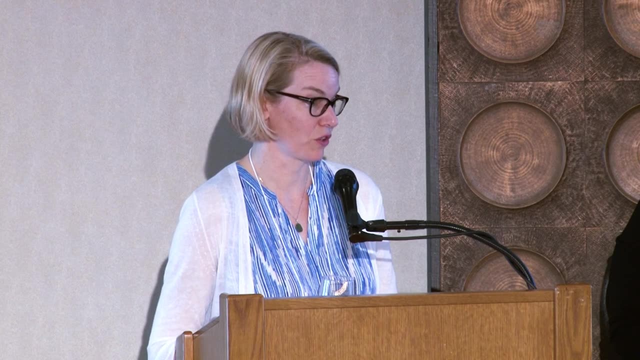 patients, And so how do we explain this? I guess I think what's going on is you're driving a whole lot of flow through very few vessels, And so, as long as your cardiac output is still in the normal range, you're really forcing. 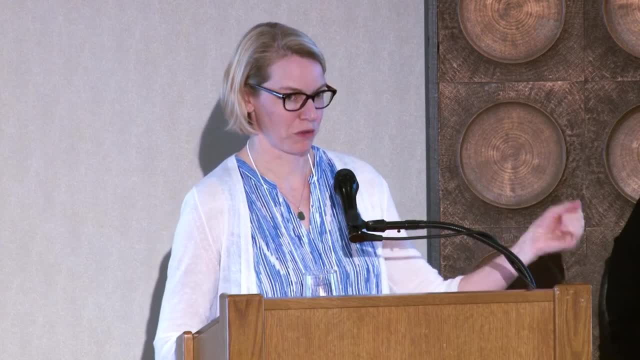 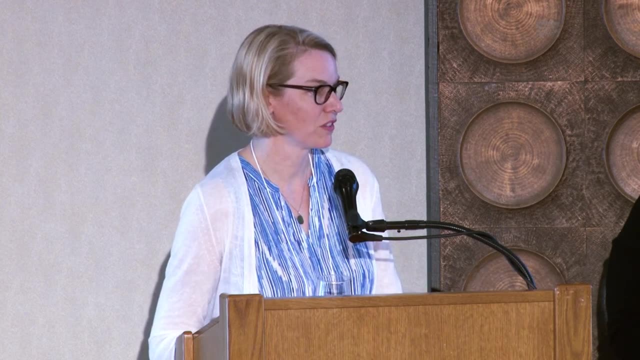 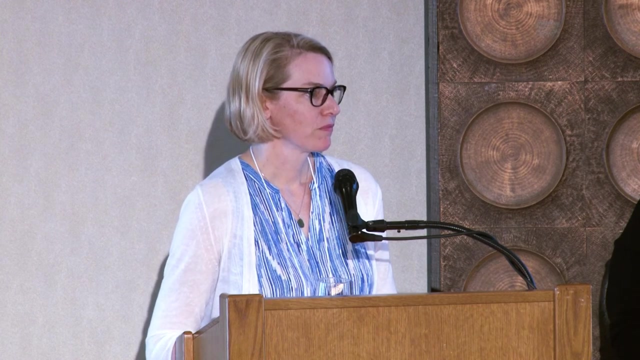 all of that flow through not only fewer vessels but vessels that are constricted, that are smaller, And so that's going to elevate the shear stress in those. I guess what I'm asking is the continuum from the as the pH got more severe. 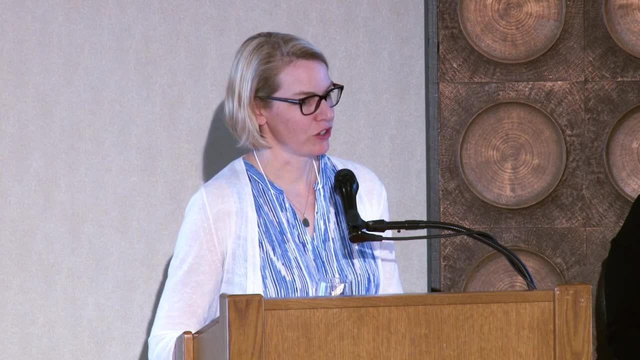 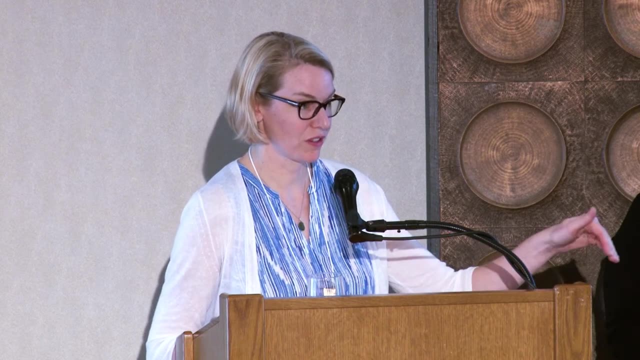 So we see, I mean, even in the normal model that I showed, we see we do see relatively high shear stress, Yeah, Yeah. So the shear stress in the distal vessels, and then that gets increasingly higher in the moderate cases and then in the severe case.